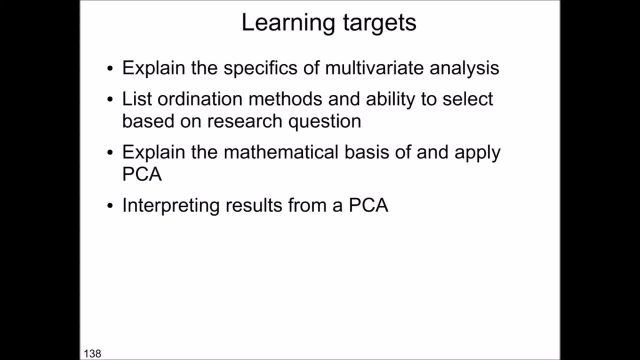 So the learning targets of today, or of this session, are, first of all, to explain the specifics of multivariate analysis, to be able to list different ordination methods and be able to pick and select favorites. random expedition200. the one that is relevant for your research question. to explain the 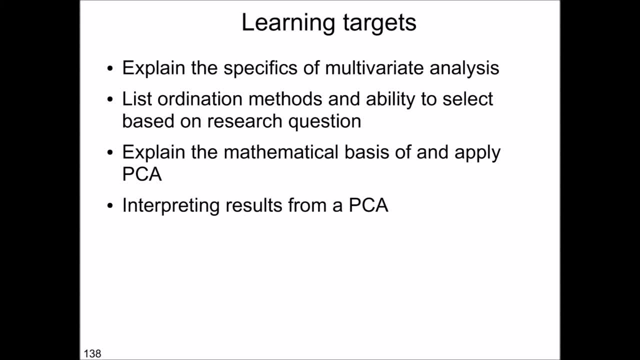 mathematical basis and to apply PCA and finally, to interpret results that we obtain from a PCA. The mathematical details are important in the context of PCA and are mainly discussed in the context of PCA and not in subsequent methods, because you understand the basis of other techniques when you understand what's going on in PCA and you will know soon. 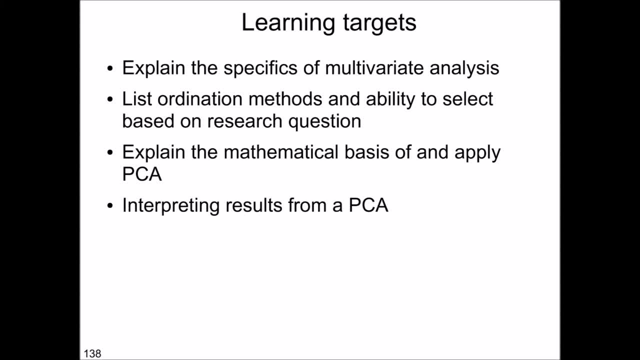 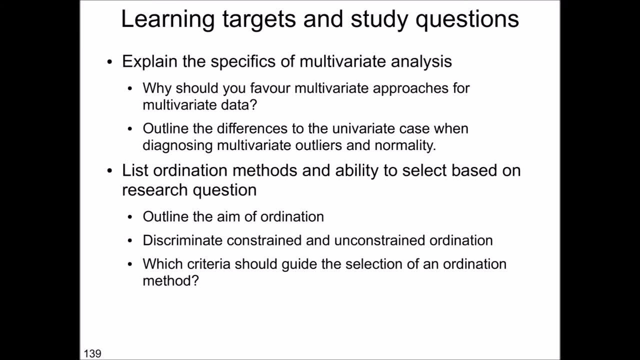 what I mean by this when you have discussed several of the ordination techniques. So here you have the learning targets and study questions so you can look at the learning targets and study questions. so you can look at the learning. So here you have the learning targets and study questions so you can look at the. 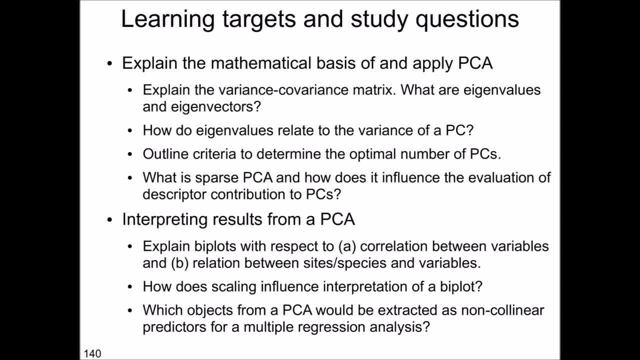 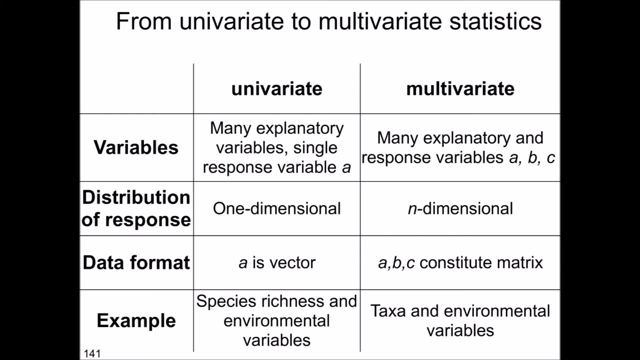 go through them yourself. yeah, additional study questions. now we start with a comparison between univariate and multivariate statistics. so in univariate statistics we had potentially one or many explanatory variables and we had one response variable. for example, we we estimated the response or we assessed the response of the predipose as well as the corroboree. 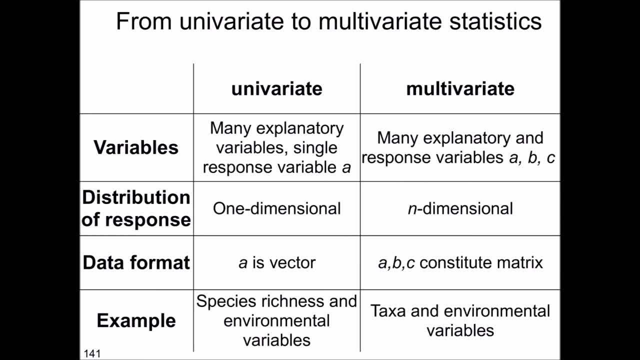 frog, two different environmental variables. so we had as response the presence and absence of the frog, and we had other topics as well, like the species richness, where we analyzed the most important variables. So the distribution of the response was one-dimensional. data format was that we had a vector and species. 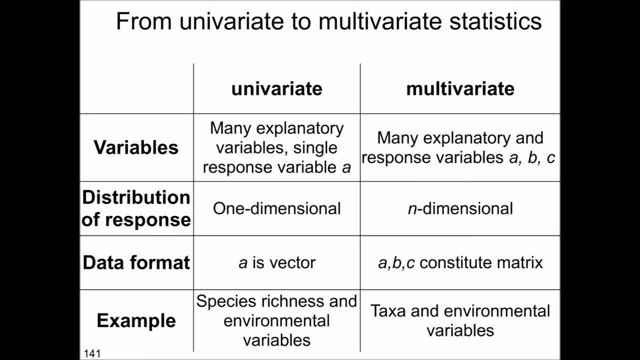 richness and environmental variables is an example for such a relationship that we had in the course On the multivariate course. this is different. we have many explanatory or potentially many. we can also have just one explanatory variable or grouping variable And we have many explanatory variables. 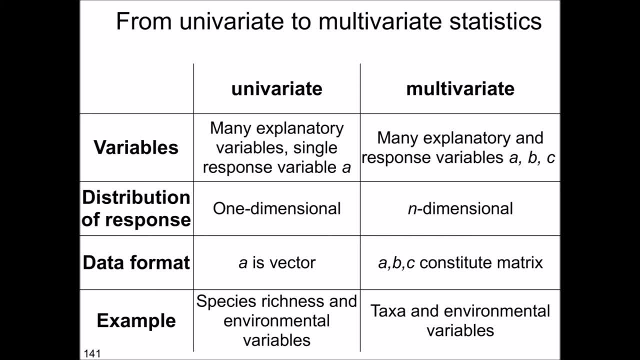 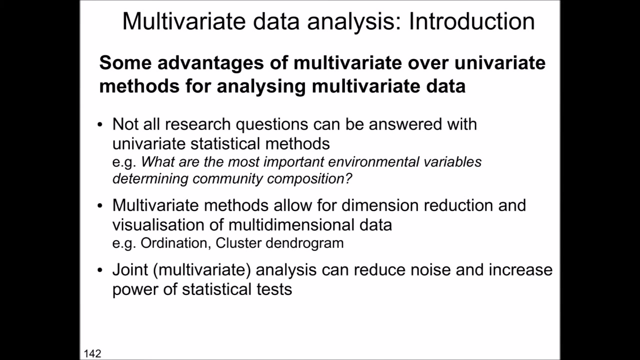 For example, we have the response variables A, B and C that are combined to a matrix. So this distribution is n-dimensional and an example is the response of taxa to environmental variables that can be assessed. What are the advantages of using multivariate methods for multivariate data? 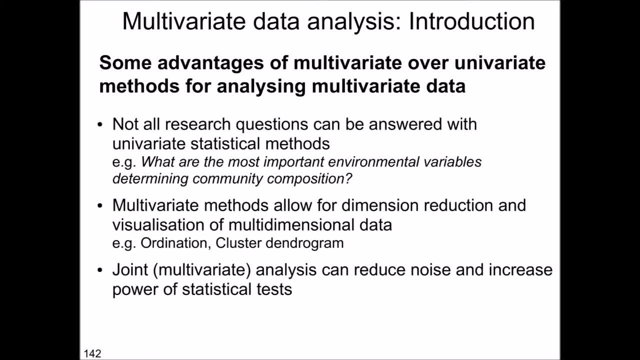 That seems straightforward, but we want to briefly discuss the justification for this First of all. I mean you could also analyze the relationship. for example, when we have multiple taxa and multiple environmental variables, you could look at the relationship for each single species and the environmental variables. 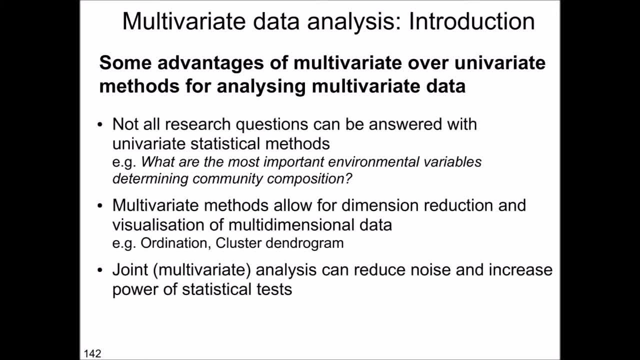 If we are interested in community response, then we certainly need to look at the relationship between the environmental variables and the whole community at the same time. So we cannot answer our research question with univariate statistical methods. An additional concern is that multivariate methods allow for dimension reduction and 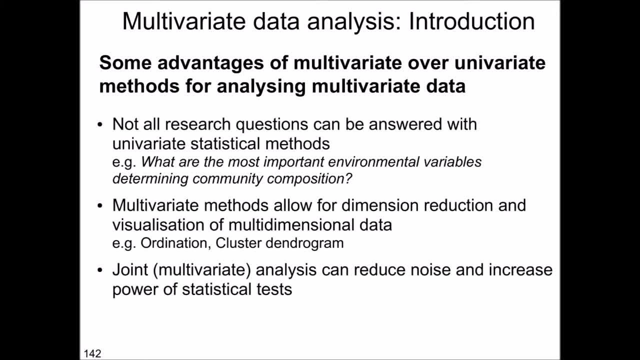 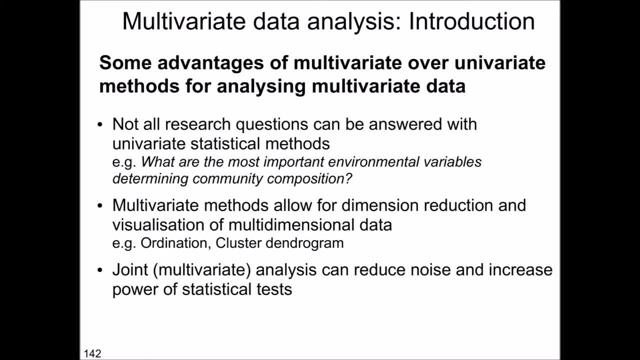 joint analysis can reduce the noise and increase the power of statistical tests. For example, we can add noise variables in statistical analysis and when we go to the, for example, we can add noise variables in statistical analysis. and then we can assume that, for example, we can add noise variables in statistical analysis and when we go to the, 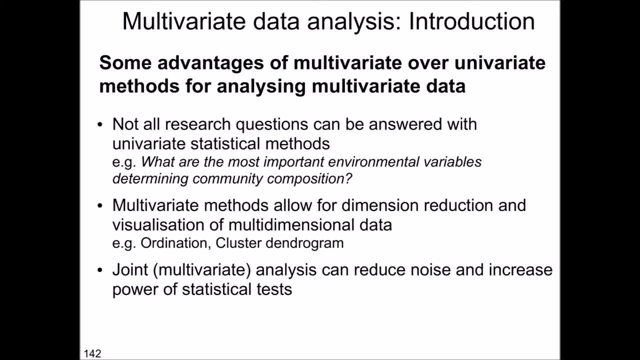 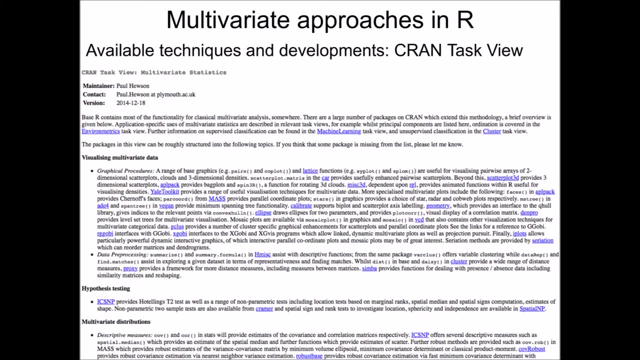 multivariant analysis. there will be a Remember, a multivariant analysis. So in time olmaz the Aqui nubes tibiali And in wine, variable analysis. of course the difference is going to be really small, given in the grand task view you can click on the slide. there's a link that brings you to the grand. 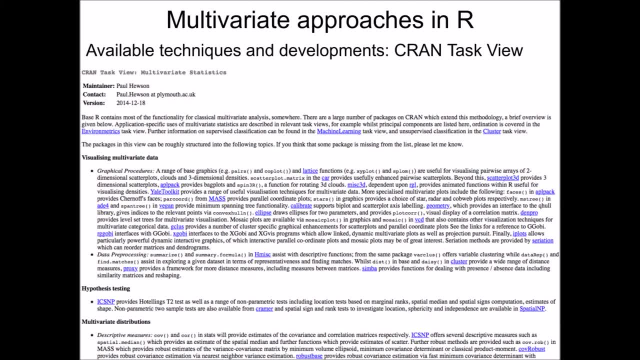 task view you get you, you obtain an overview of the different topics of multivariate analysis and the packages that that are provided. so these are many packages that are available, and task you is a little bit out of date as you um in on the slide, but it's constantly updated. 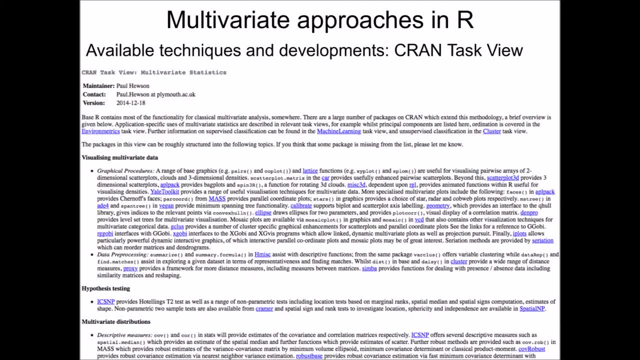 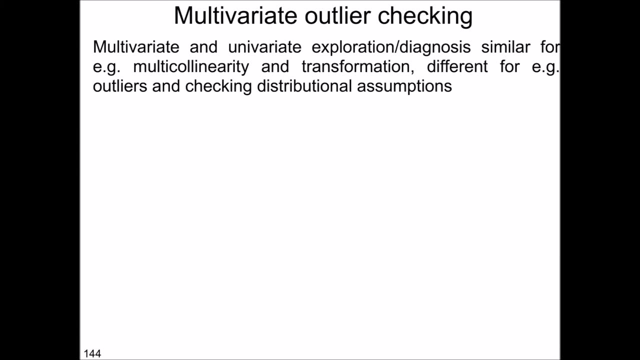 and if you want to see novel developments then look on the or forge page, and the link to this page you can find in the notes to this slide. we move on to moderate outlier checking. so several methods for exploration and diagrams are similar, between multiple rate and univariate analysis. for example, if we look at multicollinearity, foreign analysis or 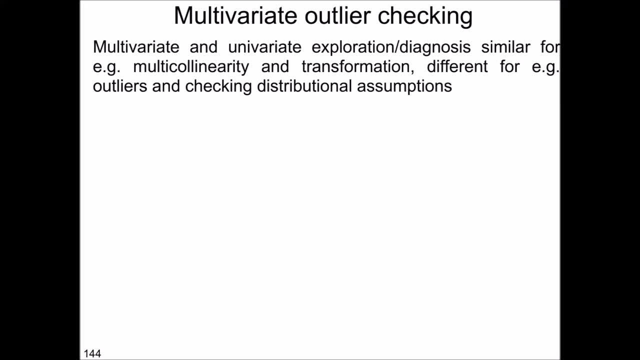 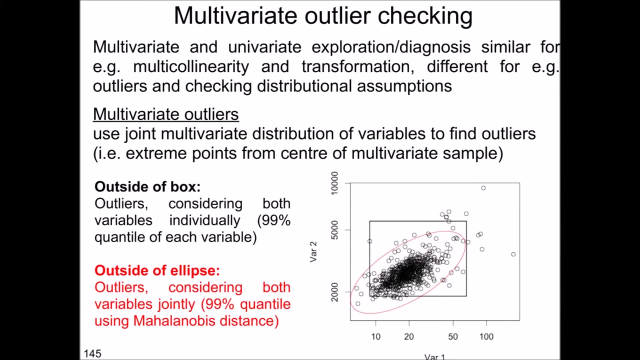 transformation of variables. but there are also differences, and we look at two differences here. this on the one hand, outlier checking and on the other hand, distributional assumption checking. regarding the outliers, we use the joint multivariate distribution to find outliers, and the difference is that in this figure here we see two variables plotted against each other, and when we just 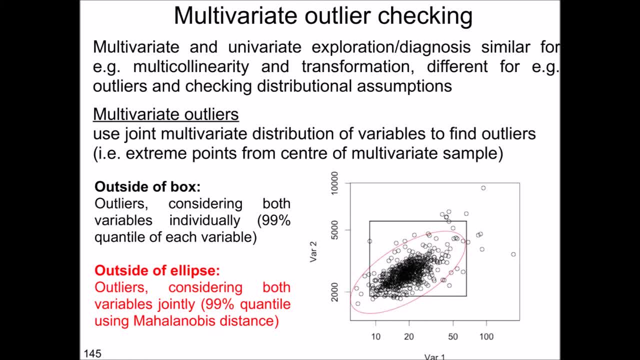 when we would just look at the outliers for one variable, then we would consider the points outside of the box, in this example, as outliers. why? because we only look at outliers that are outside of the values along one variable, so that is the parallel lines, and they form a square if combined with the, with the. 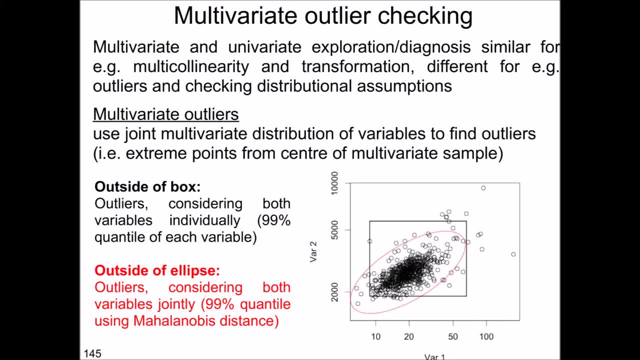 gradient with the range of variable two. however, when we consider both variables jointly- and this is done in, for example, when we calculate the model malanobis distance- i will explain later what is malan, how this model malanobis distance is calculated- then we assess jointly what is an. 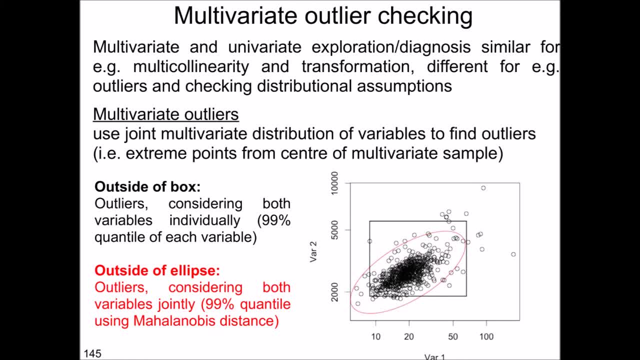 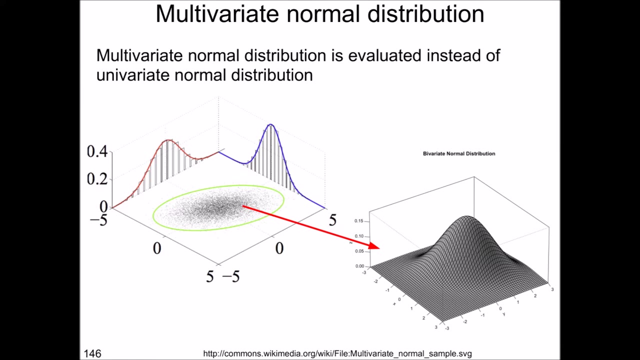 outlier and that's shown here by a ellipse that is drawn and we see that it's not necessarily the same points that would be outliers for individual variables then compared to those that are outliers for both variables. so we have a very simple distribution and we have the same distribution for the multivariate. 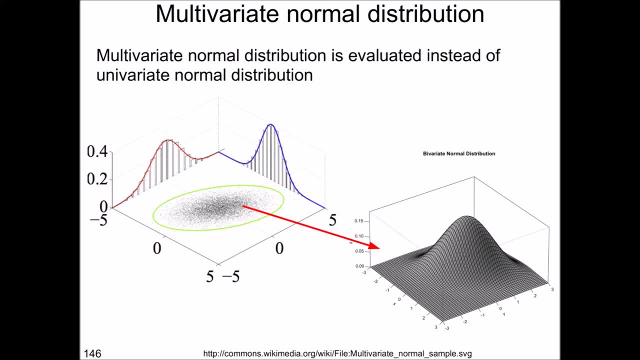 normal distribution. we see the difference here, we evaluate, and so we we evaluate the multivariate normal distribution. this is shown here for the b-variate case under. so the normal distribution in the univariate sense is shown and in the right figure and in the left figure and left. 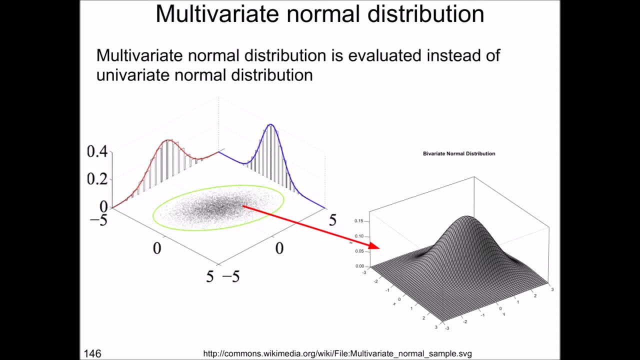 in in red and blue individual distributions and together they form a b-variate normal distribution. that's displayed in the right figure. so we draw data from the normal multivariate normal distribution. in the r example, in the r script we will do this and these data have different properties. 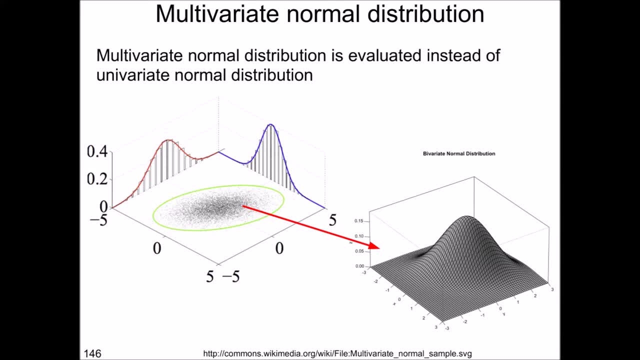 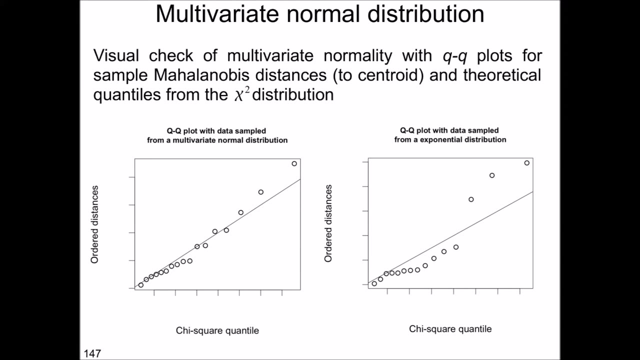 density properties than just using a univariate normal distribution. we can do this the same way that we used it in our previous example. when we look at the normal distribution, we can check it visually. what we use here is the use, the sample, non-malanovious distance to the centroid of the data. 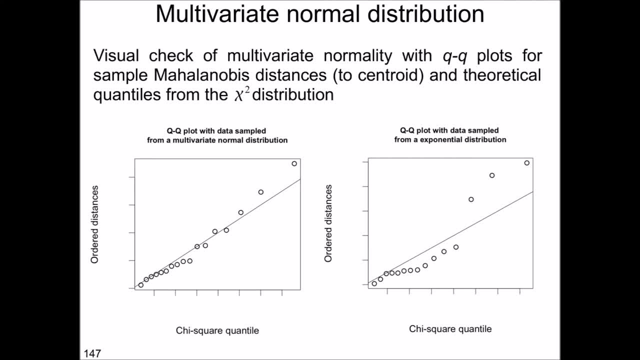 and the theoretical quanta is here- from the g square distribution, evaluate whether some data is normally distributed or multivariate, normally distributed or not. We see on the left side data that comes from a multivariate normal distribution. So there is a slight deviation. you see, for small sample sizes and on the right and right. 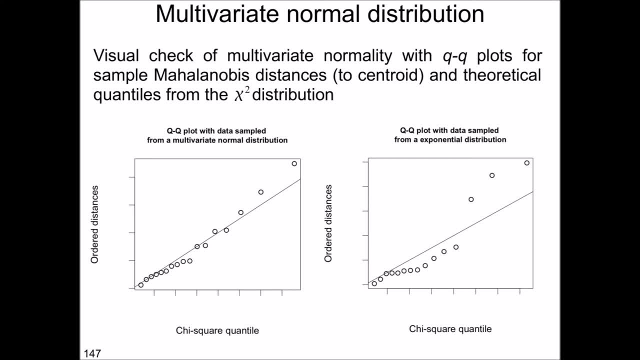 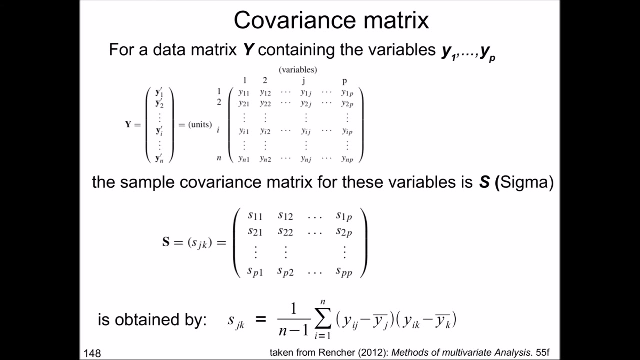 finger. you see data that has been sampled from an exponential distribution and you see that here is a quite conspicuous deviation from the normal distribution, from the one-to-one line between the ordered and the G-square distance. quantize of the distances. We have to discuss some mathematics again. 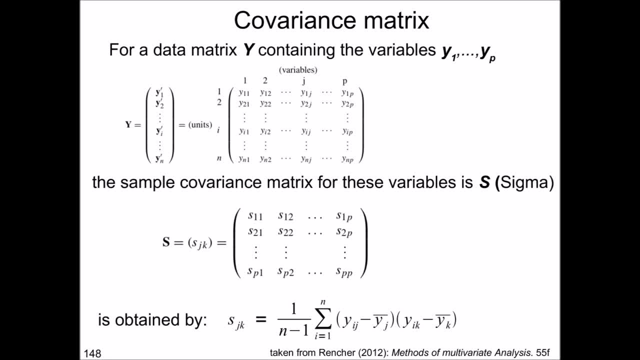 Some details In the background to understand PCA later, and one mathematical element that we have to discuss is the so-called covariance matrix. The covariance matrix contains the different variables from our data, and that contains the covariance for the variables from our data. So we have an initial data set. 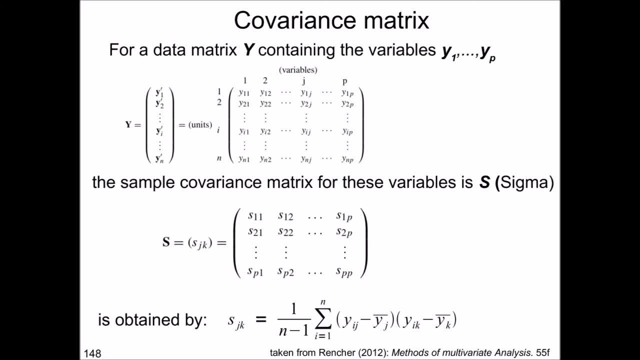 With initial data set We can have the variation of the universe by the individual variables. So you could have here descriptor variables, such as different environmental variables or also abundance of organisms. So this is this is our data matrix, and sample covariance matrix for these variables is provided. 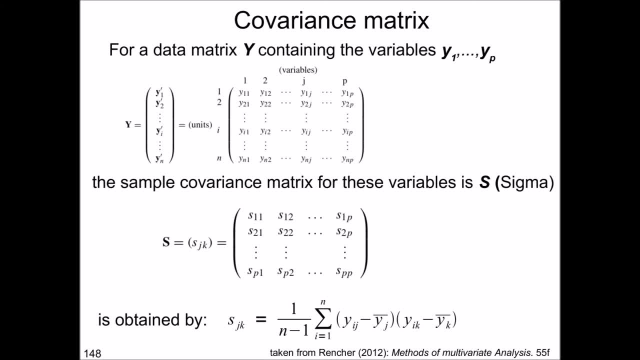 as S and you see that, as somehow it's called, sigma is smaller than Our initial. what it contains is: it contains the covariance for each of the two, of each of two variables. For example, S12 is the covariance, the covariance between variable one and two. S1P is the covariance. 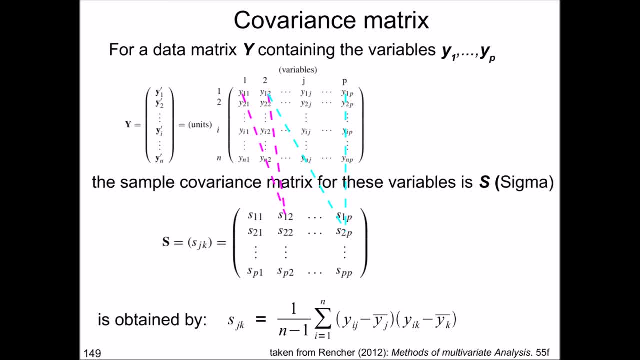 between variable S2P is the covariance between the variable two and the variable P, And here's the calculator that has shown how this is done. So it's basically we have encountered the covariance in the universal statistics context before. it is basically the covariance. 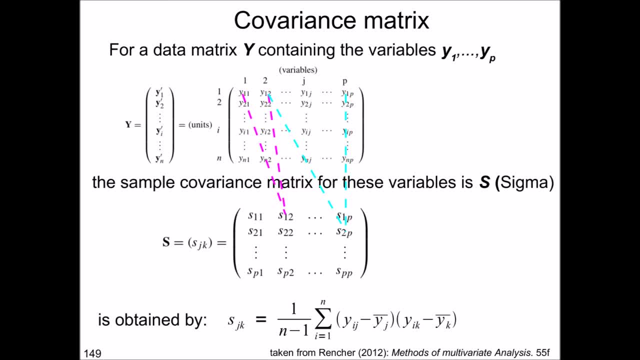 multiplication of that is given, shown in the formula here. And this is used- you should be familiar from that- from the b-variant correlation, where this is divided by the standard deviations of the two variables. This is not done here in the covariance, but there are also correlation. 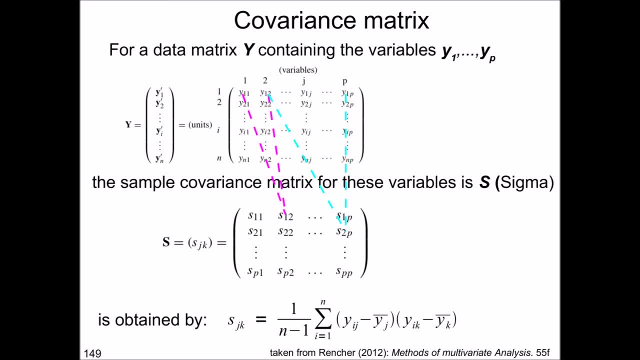 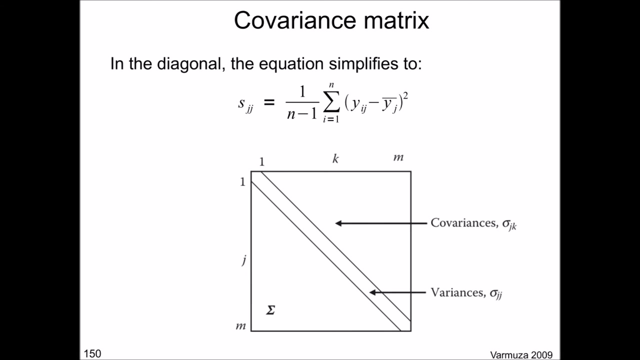 metrics and matrices where we divide the product by the standard. but we did have it in the guess that there is where we divide the covariance by the standard product of the two standard deviations of the variables. Here's another description of the covariance metrics again, And in the diagonal the equation: 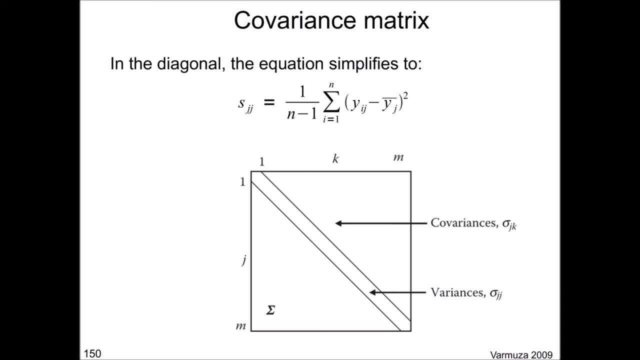 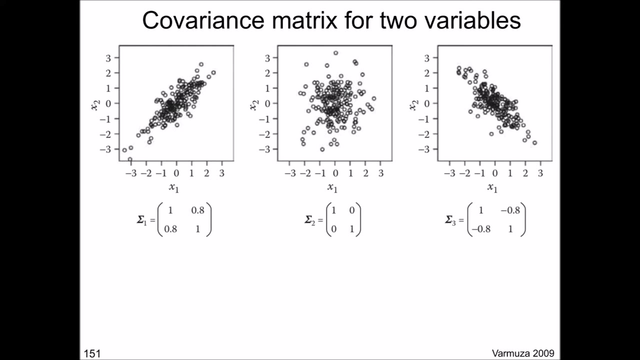 is simply the variance of the individual variables. the variables, and above and below the diagonal, have just the covariances of the two variables. Here we have a couple of plots with this, with display of the covariance we see along diagonal. that's always one. 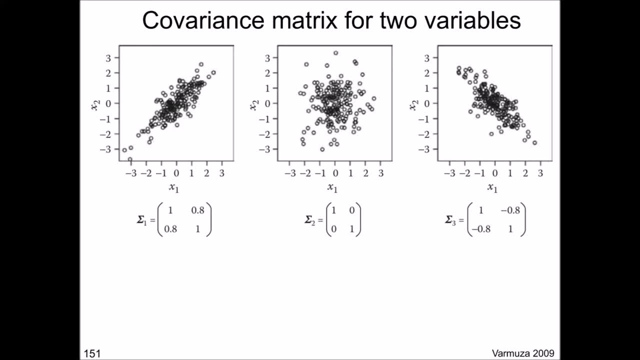 that's what we knew. the variance is one for the variables here. these are scaled variables and some scale variables. then they have a variance of one and we see that the covariance here is 0.8, which means that they are have a positive relationship. we see here the relationship is minus 0.8, so they have a. 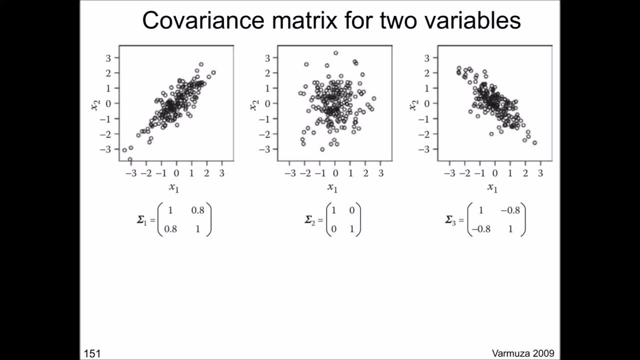 negative correlation. and if the covariance is 0, then there's basically no association between the covariance and the covariance, And if the covariance is 0.8, then they get minus 0.8. we see the outcome. So the quedarations known here are a partnership. it's single. 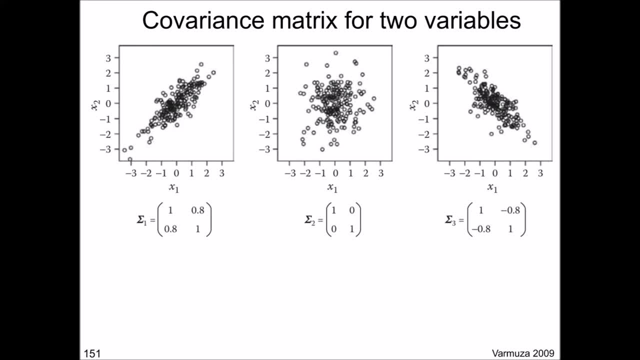 倍 and the frosting that occasionally between the two variables- distance in terms of Malnobis distance- and the calculation of this multivariate distance is shown in the shown here. so you can't compute the distance of the vector- and this is your data vector- from the mean and this is 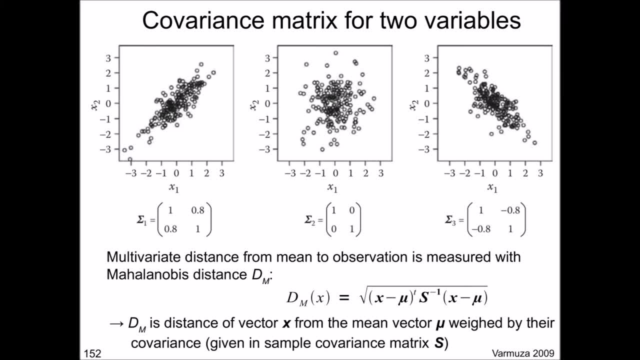 weighed by the covariance. this is given in the sample covariance matrix. so that is very similar to the set score that you compute in univariate statistics. that set score is shown. the calculation of the set score is shown in the notes to the slide. have a look at that. and the division by the standard deviation when. 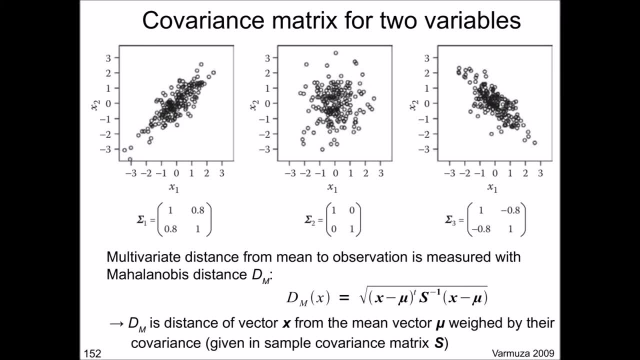 you calculate the set score has the same purpose as if, when, as the multiplication was the inverse of the sample covariance matrix, precisely to standardize the difference to the sample mean centroid by the variation in the respective variable. so we basically take the distance to the mean and then standardize this with the 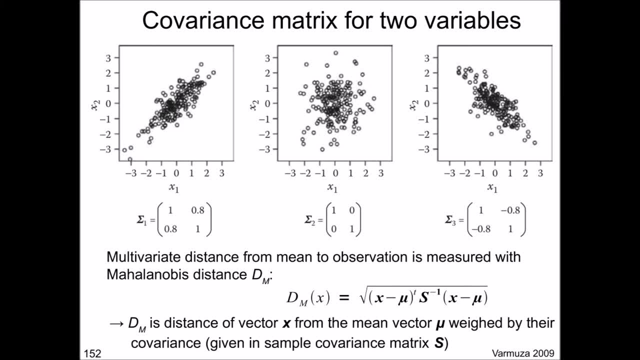 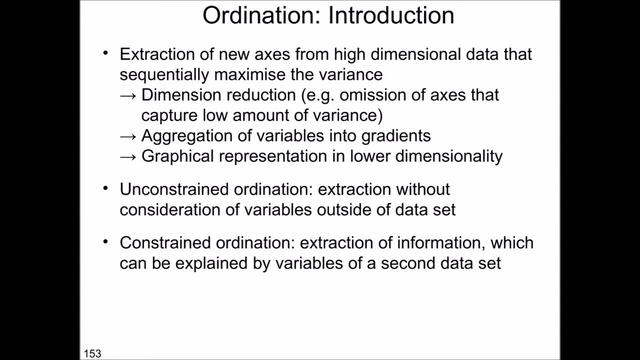 variation in the respective variable. so much about the background of multivariate analysis. some noted known notes that I had on analysis and mathematical elements that we need to understand and we move on to ordination. What is ordination? So ordination deals with the extraction of new axes from 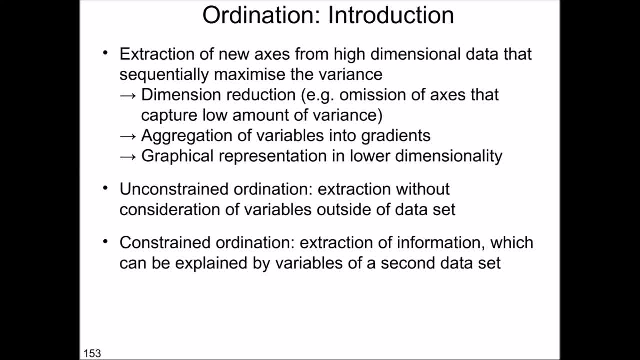 high dimensional data and these new axes sequentially maximize the variance. That means the first axis covers or captures the highest variance, the second the second most variance, and so on. So you hope that through, through this extraction of new axes, the first few variables and axes that you extract capture the major part of the whole variance in the data. 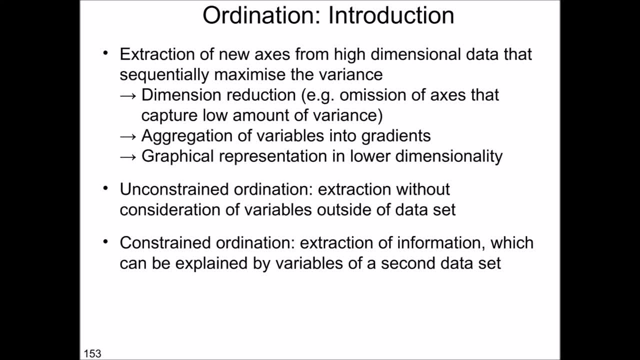 That is especially the case when there is a collinearity between the descriptors in the data set. So you could theoretically achieve dimension reduction by omitting some of the axes afterwards that capture only low amount of variance. I will give notes of cautiousness on this. later on when we discuss Principal Component Regression, You could use it to 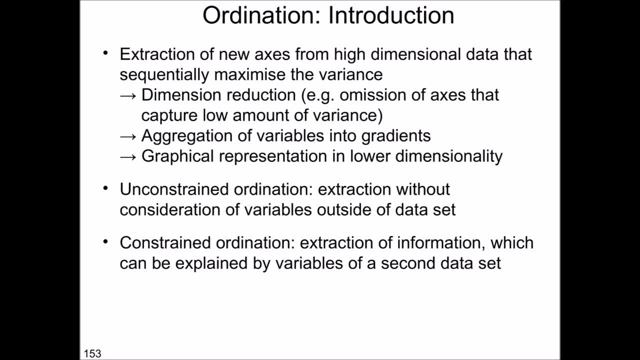 aggregate variables into gradients- We'll see later on what I mean by this- and you can achieve a graphical regression according to your theory. if provisions within a certain menus are Bears Variables in a customer set with relatively high gamma values and kept, make a variable in a advanced 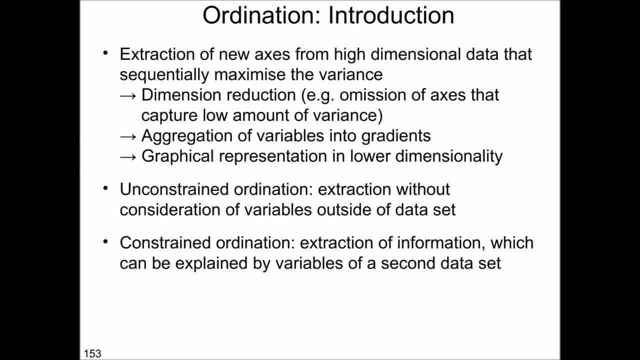 uhh mode. Inclusion usually belongs more to a product which would be defined by some couples regardless of the client. You could use it to painstakingly estimate the time frame of the categorization, presentation and low dimensionality, as discussed before. we can't display four axis or four. 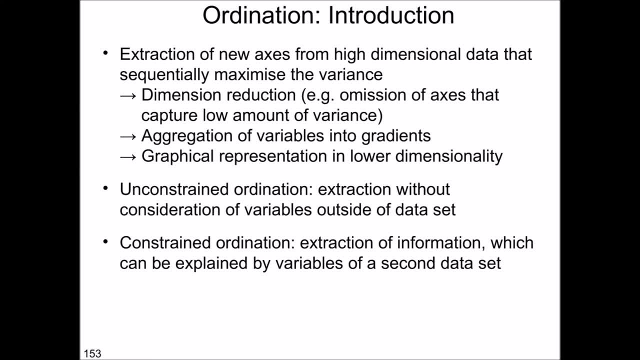 dimensional data at the same time. but if we achieve to did to capture most of the variation in our data with two axis, then we can easily display and visualize this. there are a couple of papers on multivariates methods with focus on ordination and you should have a look on. 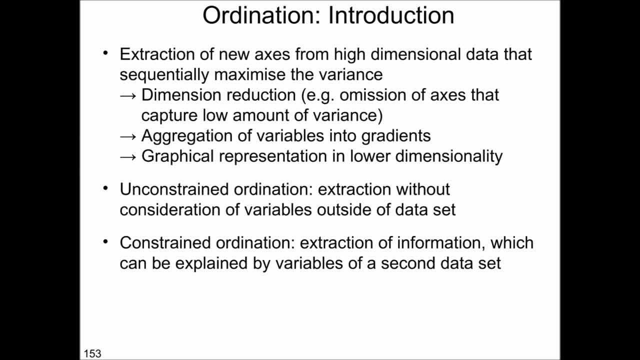 the notes, in the notes to the slides, where i give you several paper links, and most of these papers are freely available. so there are two methods of ordination that you should be familiar with. the one hand is unconstrained ordination. you should be able to explain what. 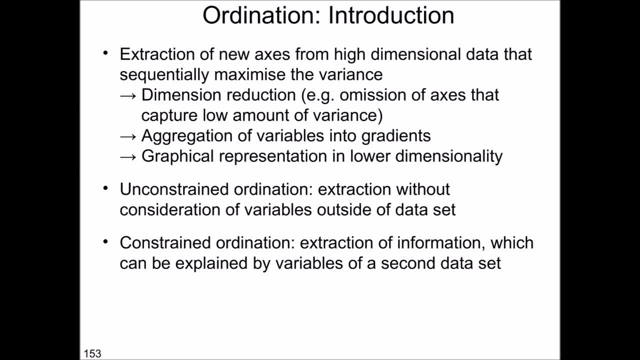 it means? that basically means that you extract the data from your data set without consideration of variables outside of the data set. so that means to just take your data set and you run the ordination- constrained ordination. you extract information in your so-called response variable data set, then with considered by taking into account explanatory variables from a second. 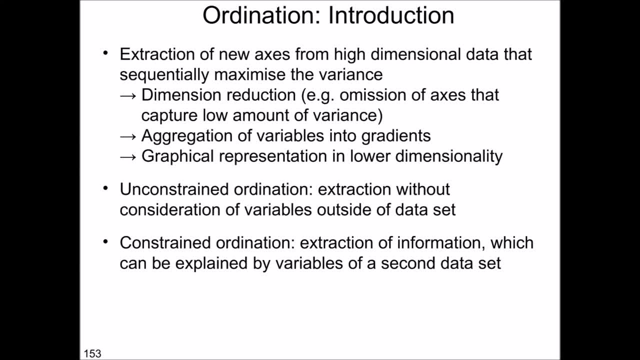 data set, or that would be the case if, for example, you want to explain the response of organisms to the environmental variables. that would be a constrained ordination case. so you take these environmental variables to extract information, species information, whereas if you just look at the relationship between sites where species have been observed, so which sites are similar? 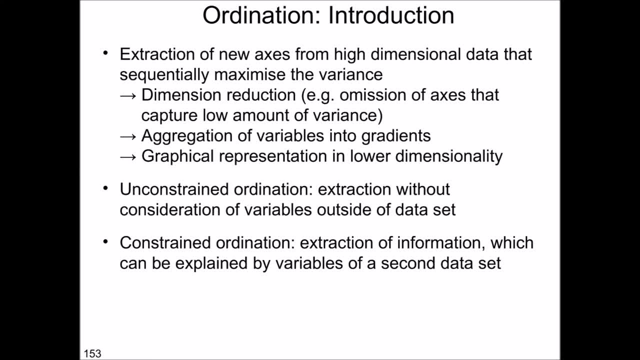 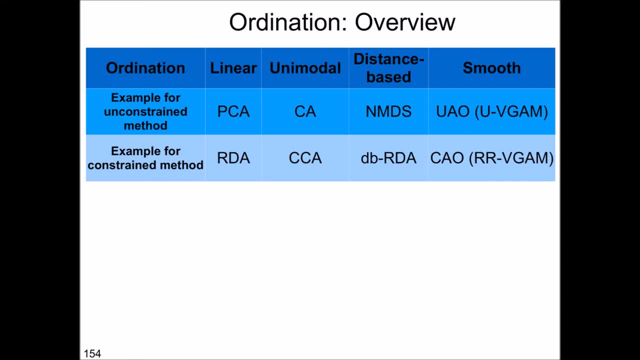 then you just use the species data and that would be an unconstrained ordination. so here you have an overview of the different ordination methods. we don't have time to cover all of these methods in the course. these are examples of prominent methods that are used. 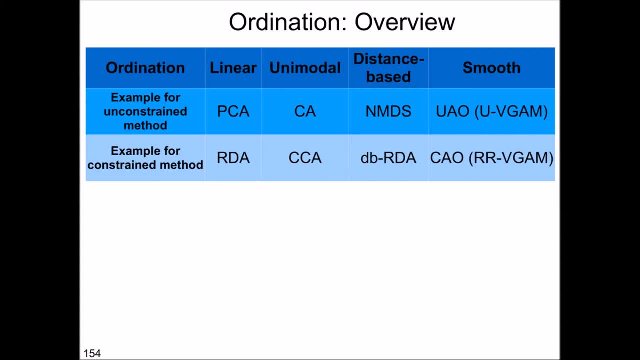 used in this context and we can classify them by how they deal with the, with the distribution of the data. if we have linear relationship in the data- so this is displayed on the next slide as well- then we use, can use a pca if we have linear gradients. if we have rather unimodal gradients, then we can, should use a unimodal, then we should. 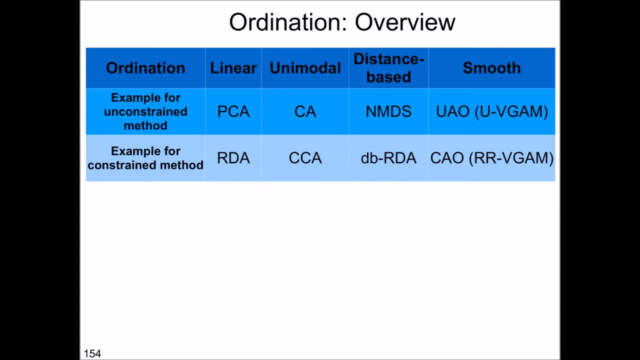 use a correspondence or analysis or different methods that capture these types of distribution of gradients, distance based and, finally, smoothing techniques that rather are data driven than model driven. so we don't assume a certain certain distribution of the data or shape of the data, but we just fit. 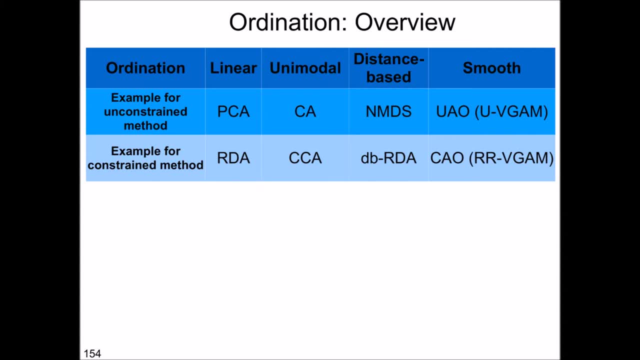 a shape from the data itself. so the different, what these different acronyms mean, is also stated, and this and the notes to this slide. have a look there. first we have the unimodal gradient. so we see the species density increases and then against the environmental variable and then decreases again. that is a unimodal relationship. 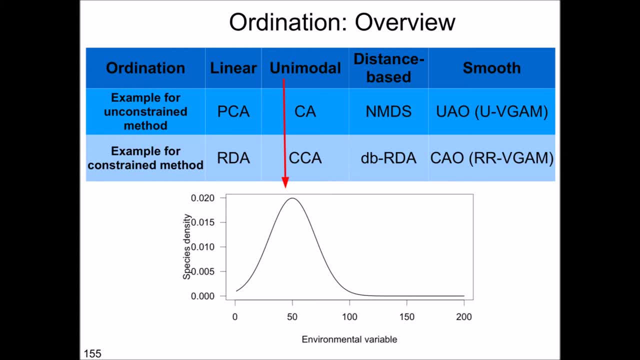 between the response and the environmental variable. of course you're only shown for the, for the b variant case, the linear relationship. we would just look at one part of the environmental gradients. so along the environmental gradient we just have an increase of the species density, and distance-based methods capture various relationships between the. 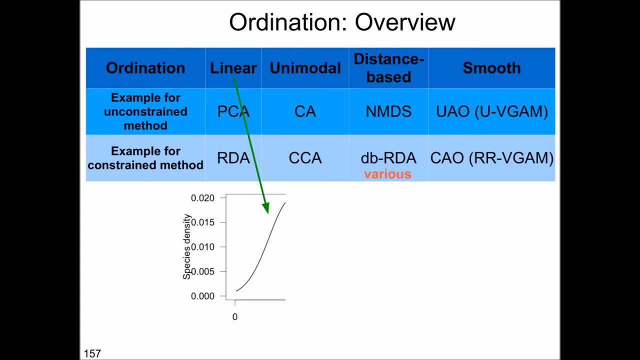 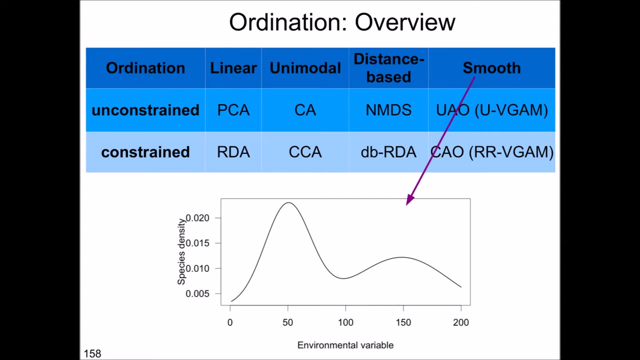 species density and the unimodal gradient. so we can see that this is an unimodal gradient which can be used to determine the relationship between species density and the environmental variable. so they are relatively flexible. and finally we have the smoothing techniques. we see here an example. 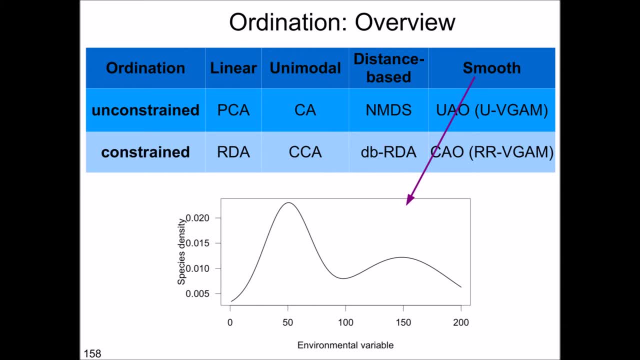 how the smoothing technique can capture species density that are neither linear or uni-modal. we have two peaks against the environmental variable, so this is well captured by such data driven techniques. so, depending on the assumed relationship between the environmental variable and your your response variable, you should select you. 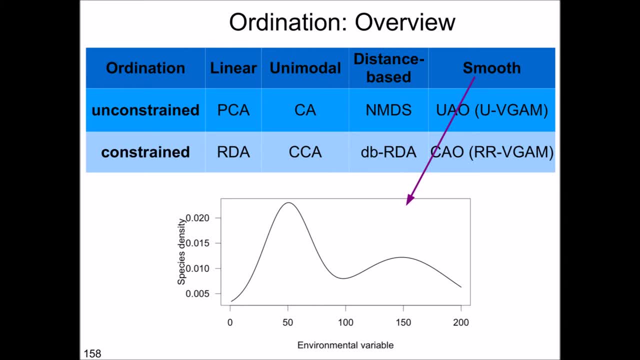 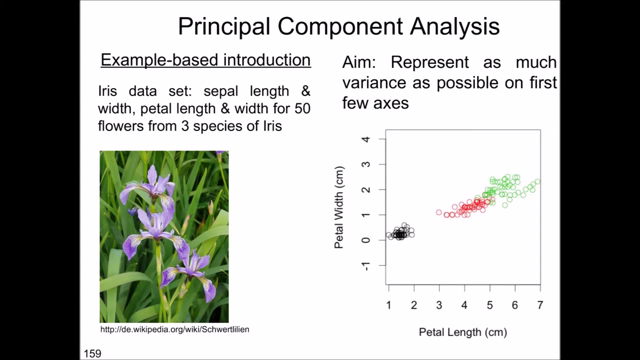 you should adjust the selection of the ordination method you. so we turn to PCA now. PCA is principal component analysis, and we do this with an example, the data for this example is a famous virus data set. so these flowers: you see a picture of these flowers and four variables of these have been 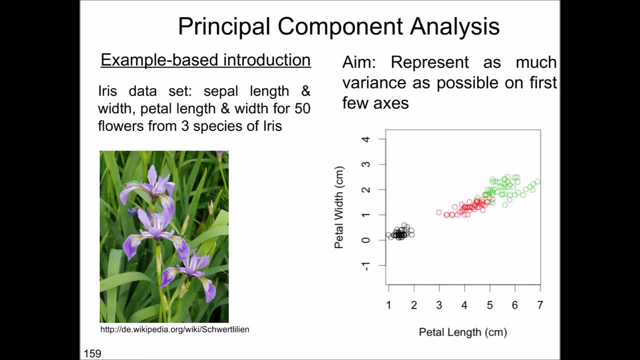 measured on the one hand, the sepal length and width, the petal length and width, 450 flowers from three species of iris and you see an example plot here on the right side on the figure. that's the petal width against petal length and we see here the three different species are all indicated with different colors. 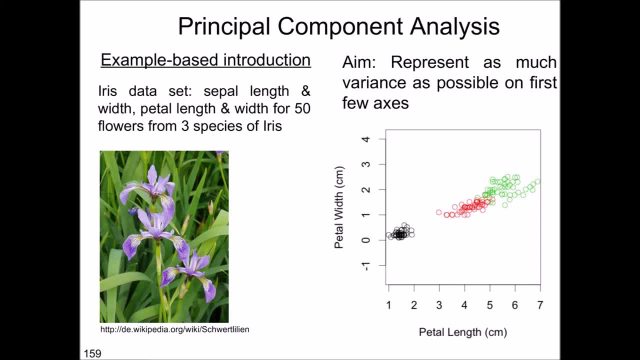 So what we do is, when we do this in this introduction example base, our aim is to represent as much variance as possible on the first few axes. So the first axis should have the major variance. So the number of axes is always the number of variables or descriptors in the PCA data set. 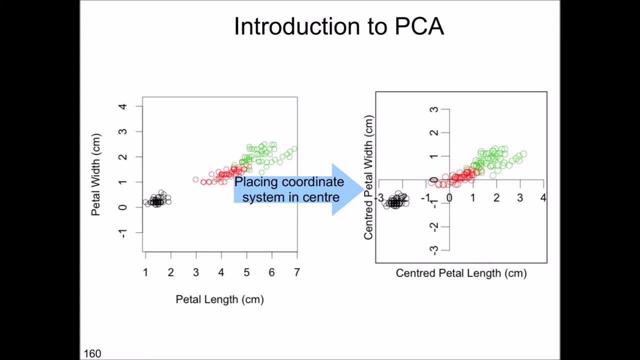 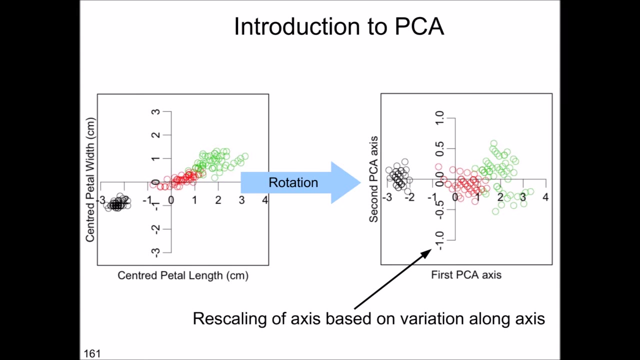 So the first thing we do is we place the coordinate system in the center of our data. So we center our data that's displayed on the right hand side, and after we have done this, we rotate our coordinate system to a heave that the maximum variability in the data is along the 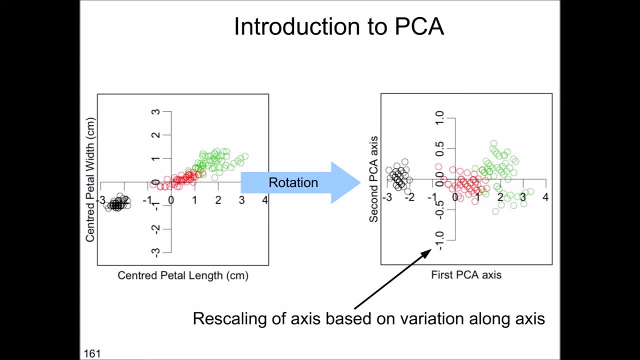 first axis. You can already see this in the left figure- that if we slightly rotate the axis, then we have a much higher range along the x-axis compared to the y-axis. And what we do as well is we rescale the axis based on variation along the axis. 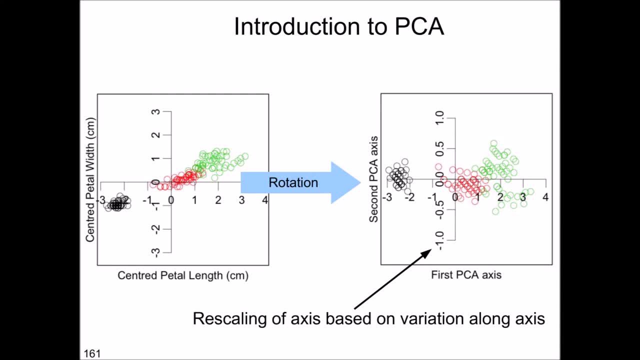 So we see here that before the scale of the y-axis was from minus 3 to 3, so it had the same scaling as the x-axis, So one unit was the same in both dimensions. Here we rescale that the axis ranges from minus 1 to 1, and this is done to achieve a clearer 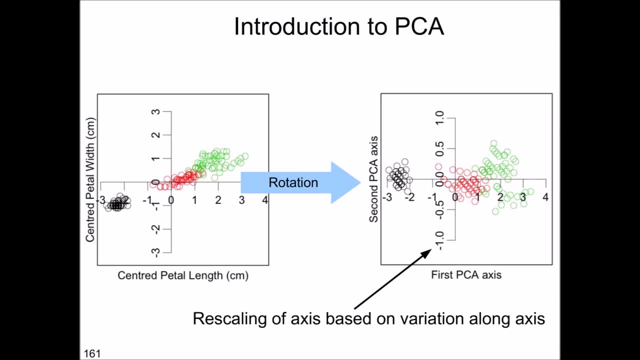 separation between the points along the y-axis. So one unit at the distance along the second axis is not the same distance as along the y-axis, along the x-axis. so that's important to understand generally in ordination methods that the differences at the distances depend on how much of the variance. 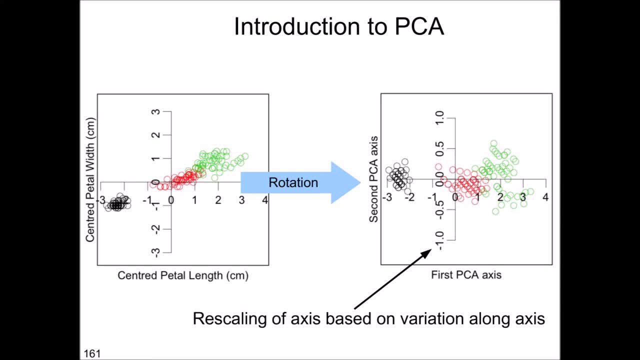 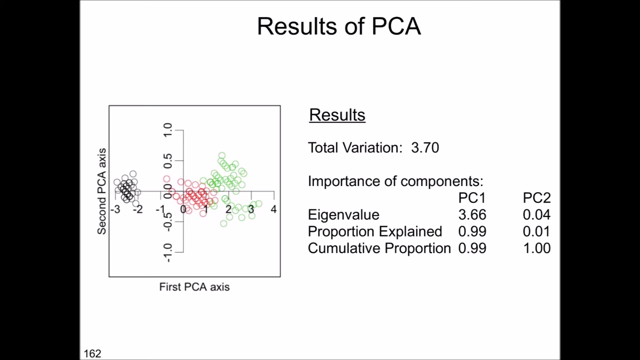 is captured along one axis, So we won't discuss scaling in detail in the course, but there are different ways to scale the axis, And this is described in the literature and in the R vignette to which I referred you to. What we obtain out of the PCA is then this plot: 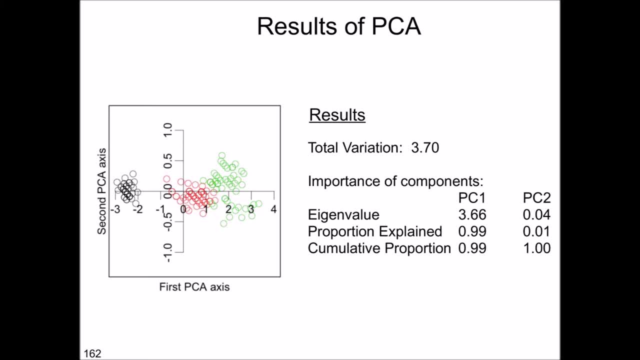 So we have a separation of the data and we can. this is a way of visualize the relationships between our objects and, on the other hand, we have some results on the right hand side of this slide and, for example, the total variation of the data. that is, the total variance, and we obtain information on the importance of components. 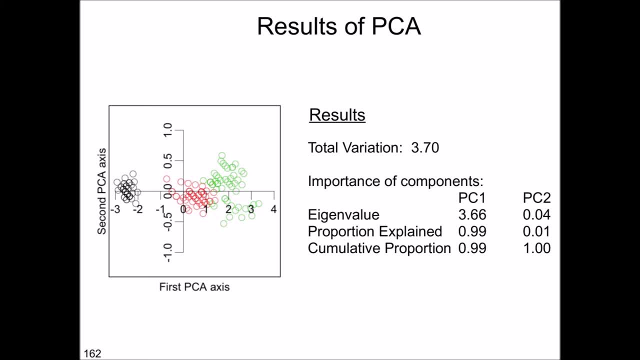 in the one hand, and these are the so-called eigenvalues, the proportion explained and the cumulative Proportion. that sound may sound a little bit difficult for you at the moment, but you will understand these terms later on. Yeah, the total variation is clear: it's 3.7. if you would calculate the individual variance for 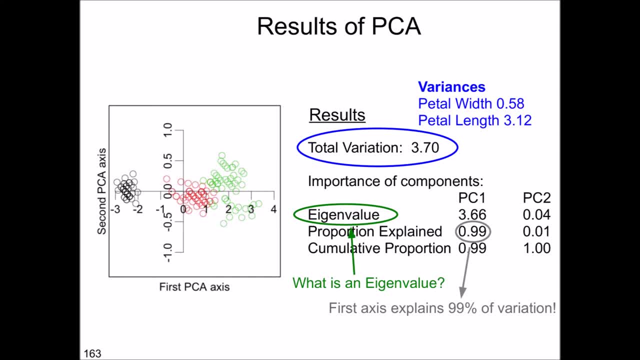 petal width and petal length, we would see that the sum of these is 3.7. that's how we obtained it. Eigenvalues are explained later on and we see that the first axis explains 99% of variation. So if we just look along the first axis, we would already capture most of the variability. 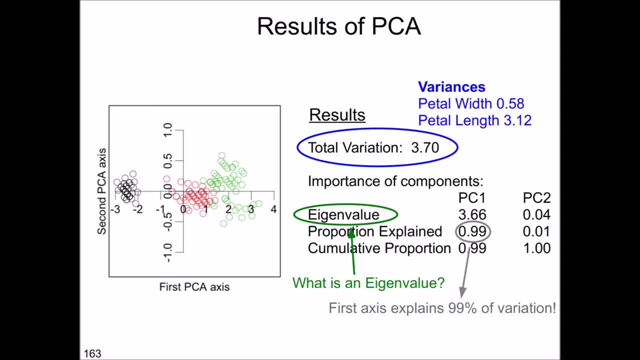 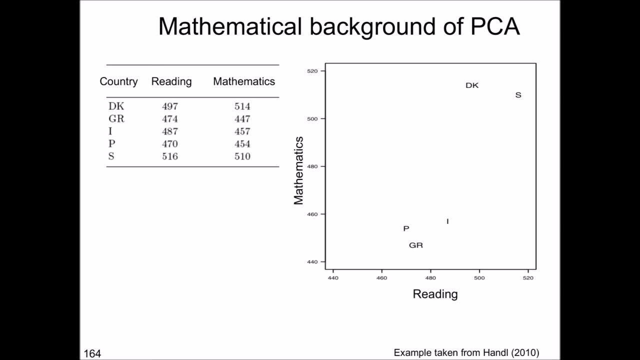 in our data set and we could interpret the relationship between objects, for example sampling sites, by just looking at the distance along the first axis. And we already have 3.7 that we need to translate in the next iteration of the row by 2-3-5.. 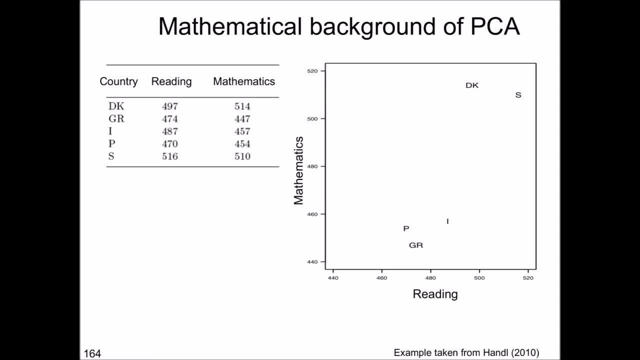 However, we want to understand what's going on mathematically in the pca and we do this by choosing an example, namely the PISA study, and i choose this because this has been nicely displaced in displayed in the literature. have is: initially, we have some scores and mathematics and reading. you know. 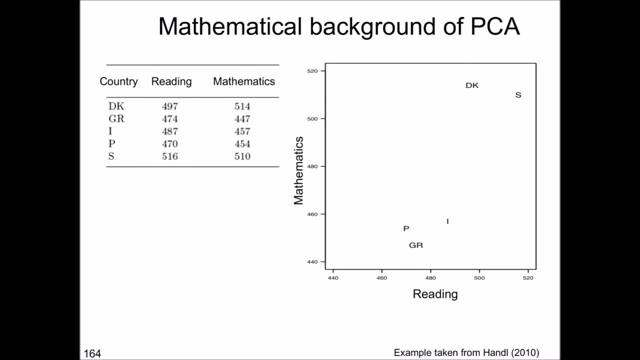 that pupils are ranked in PISA according to their performance in different areas of education. so here we have mathematics and reading, and we have five countries for illustration that have different points. so our aim is now to we start first by centering the data, as before. so that is shown here by the red cross on. 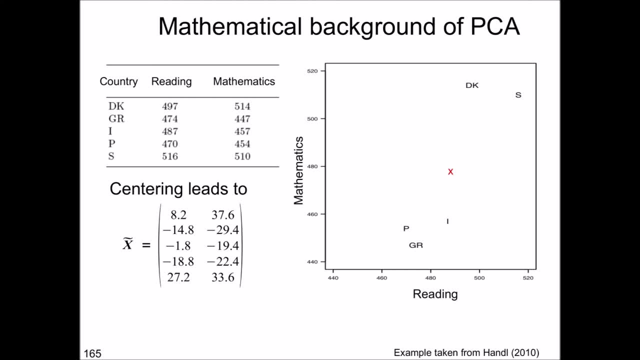 the figure and you see the send, the matrix of the centered variable. so we have the this tilde on top of the variable. that indicates that we have an estimate instead of an head. so in the context of multiple regression analysis you had, you had an X or Y head, so here we have a tilde that indicates it's an estimate. 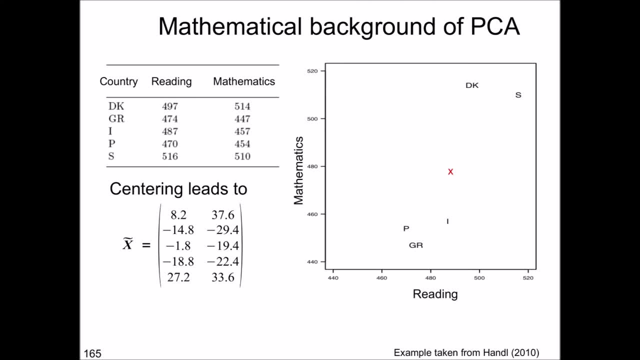 for transformed variable because the centering reprints represents a transformation. so centering changes these different points. you changes the points. you don't need to scale the variables here because they are basically on the same scale and our aim is now to search for the first axis with the maximum variation in the data. that's. 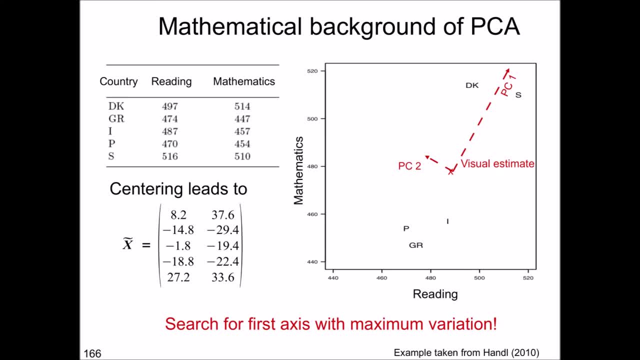 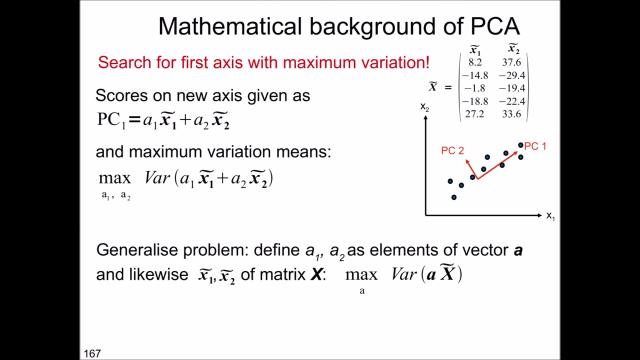 shown here in these dashed lines in the figure. that's just the visual estimate how the PCA one day first PC accessed and the second principal component will look like. so let us translate this search for the axis with the maximum variation into something more palatable. we have scores. 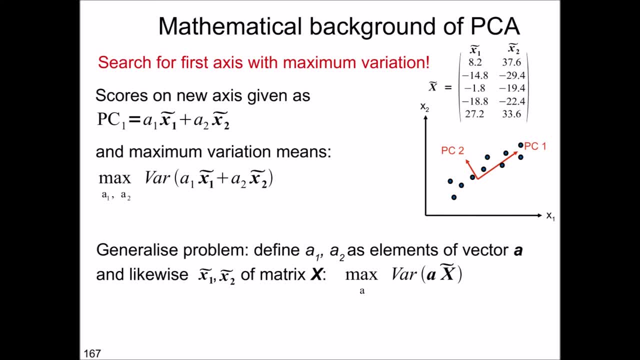 these scores express what the coordinates are of the initial transformed objects on the new principal component axis. so for principal component axis one, just let's focus on this case- here we would have the initial coordinates with the center variable X 1 and X 2, with a tilde, and to obtain 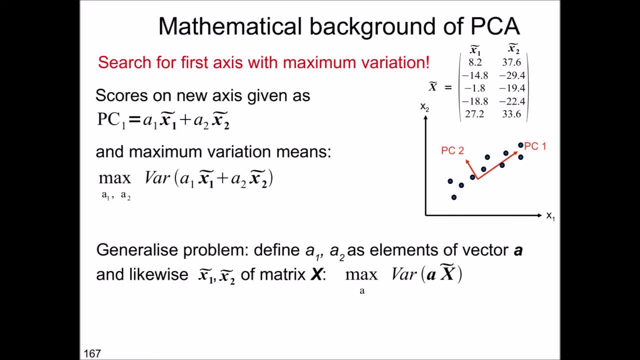 the new coordinates, we would need to multiply them by two unknown factors, by two unknown variables, a1 and a2, and this will result in the scores on PC1. Now, what does mean that we've looked for the maximum variation? we need to have an argument of these score. this scores that. 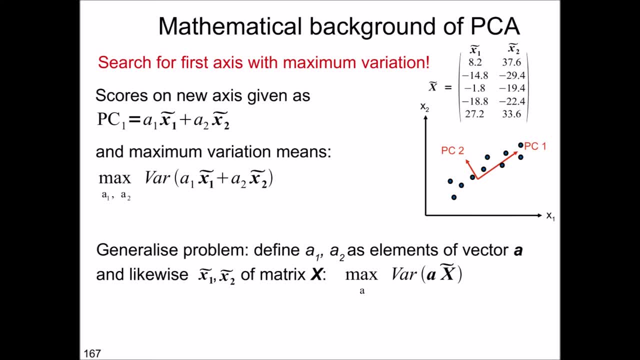 we search for the maximum variants: a1 multiplied x, 1 estimated transformed variables, x1 and so on. we can generalize this problem, and a1 and a2 are elements of alemtics. more than once this has been the rule orкольку. we can then sentence bad values: x, u and c ox. 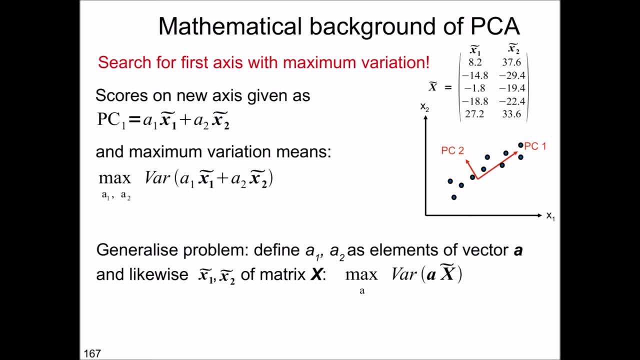 a vector. These vectors we will later call eigenvectors and we consider that x1 and x2 are elements of the matrix X and can rewrite this whole problem as maximum of A is the variance A times the matrix of transformed variables, the centered variables. 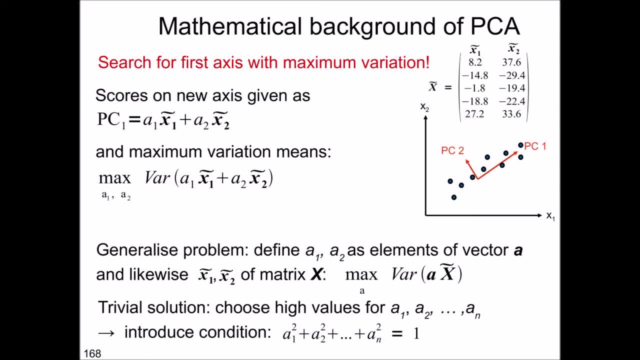 Now a very trivial solution would be that for the individual elements in this vector we choose, so in the eigenvector we choose just very high values, because obviously if we choose very high values for A1,, A2, and so on, then we obtain a very high number of values. 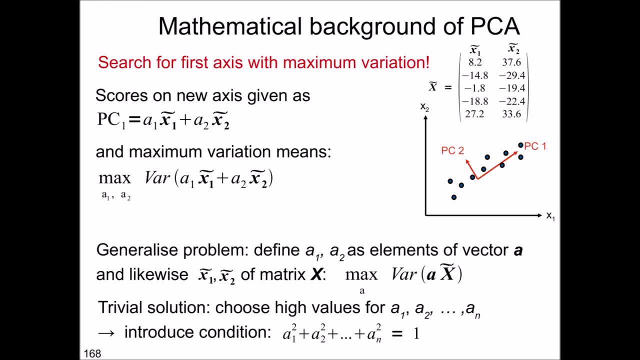 So if we choose a very high number of values and we inflate the variance, so we need to somehow introduce a condition that limits the value that we can put for A1, A2, and so on for the individual elements of the eigenvector. 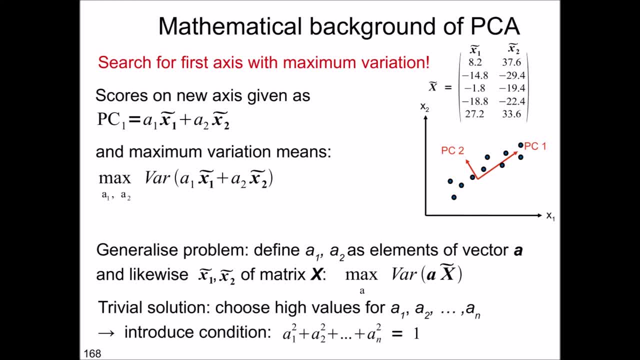 And we say that the sum of the squares of the elemental of the vector should not exceed one. So this is shown here by the introduction of the condition For the Pisa example. just imagine we set different A1s and A2s. 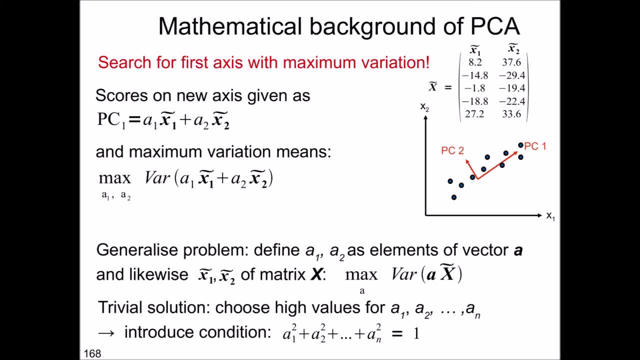 So the value of A1, with which we multiply x1, and the value of A2, with which we multiply x2.. In the example we could, for example, set A1 to 1 and A2 to 0. Then we obtain just the variance for x1, because xA2 is 0. 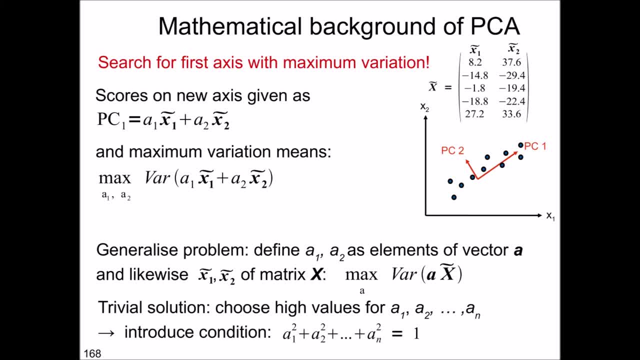 If we set A1 to 0.6 and A2 to 0.8,, this would be another set of variables that yields to 1 that meets the condition of 1.. Then we find a certain variance And we can choose different tuples of values that have an if squared and summed up, yield 1.. 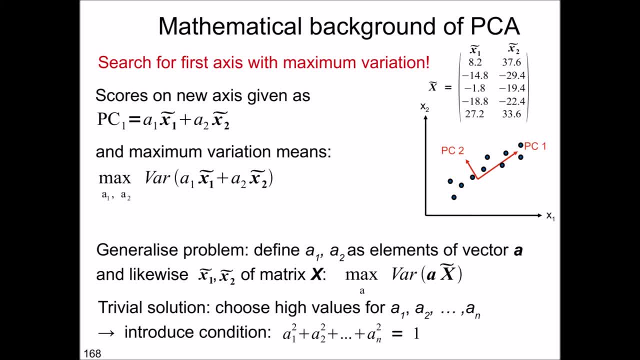 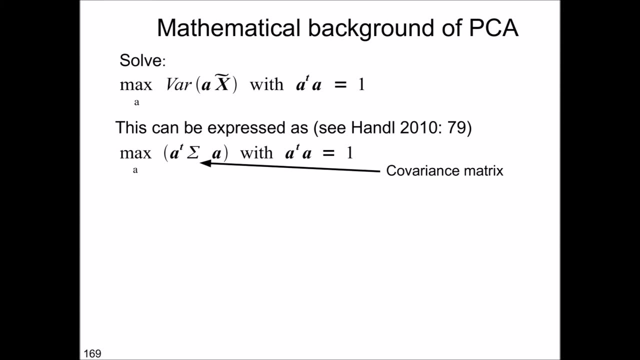 And we need to find that one that maximizes the variation, So that has the maximum number, maximum variance here. The ideal variation in this case is a set of a primary training, set of A1 and A2.. A1, a variable between A1 and A2.. 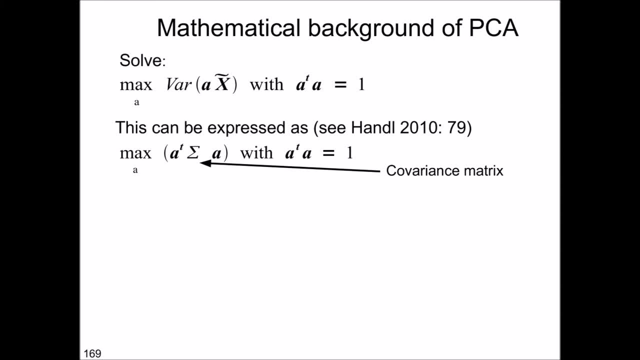 So expressed differently. we searched for the maximum variance of the problem of A multiplied with the matrix, under the condition that the vector A multiplied with with the transposed vector equals 1.. In this case, can be expressed as in a different form because the the transcended matrix of transformed values. 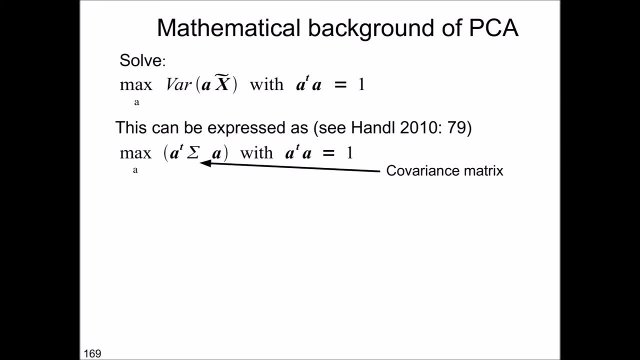 when we search the variance for this, we can just use the covariance matrix here and we multiply the covariance matrix with the, with the transposed vector of a and again with a, under the condition a, t multiplied a equals one. now maximizing an argument you may notice from different fields of science. it's, for example: 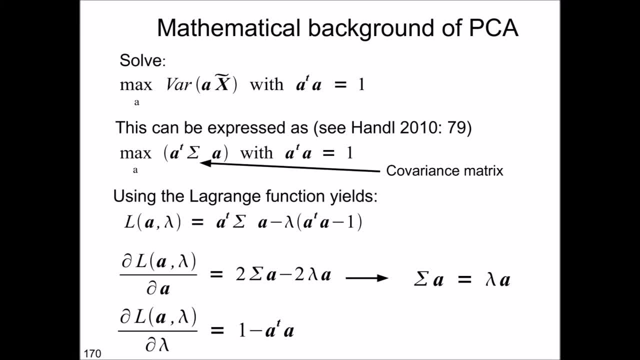 used in economics as well, why you can use a lagrange function to maximize the to to implement this function and as when we implement both conditions into this function. so we choose the first part: 80 multiplied with the covariance variance matrix, multiplied a minus lambda times, and then we have the condition. 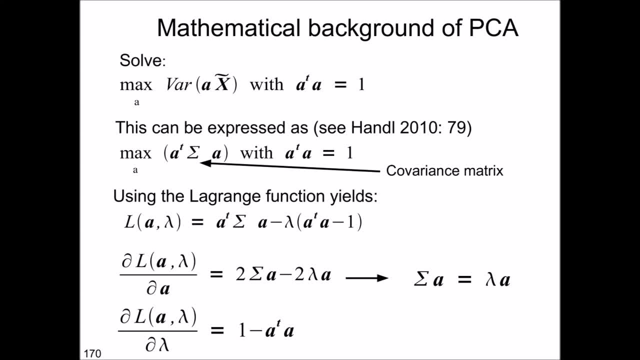 that the vector multiplied with its transposed should yield one implemented and in the brackets. so now that we want to maximize, we look for, we differentiate to find the peak of this function and we differentiate for, for a, and if we do this, you see here on the 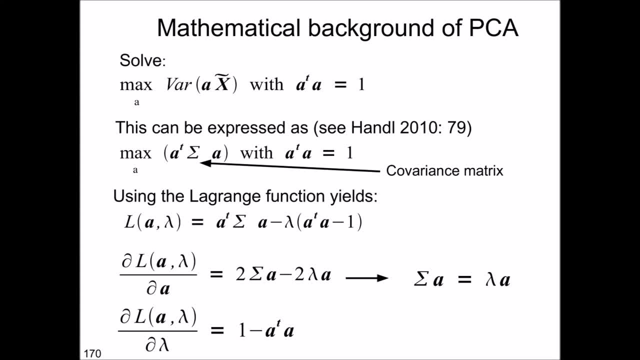 on the top and on the bottom. second equation: from the bottom you see differentiation for a and we see that two times this covariance matrix multiplied was a minus two times lambda, times alpha and minus times r a and this can be reformulated to the variance covariance matrix multiplied. 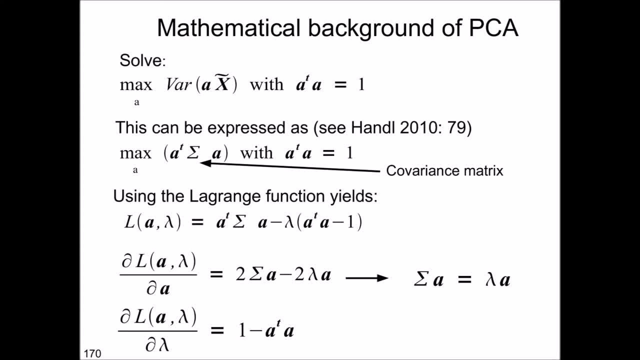 with a equals lambda times a, and this is in fact the so-called eigen value problem. and this is the eigen value problem, and this eigen value problem where we will discuss in the next slides in general form, not specifically in the context of pca, but you need to understand this. 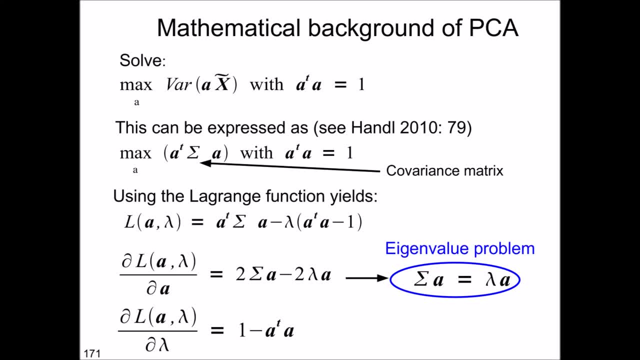 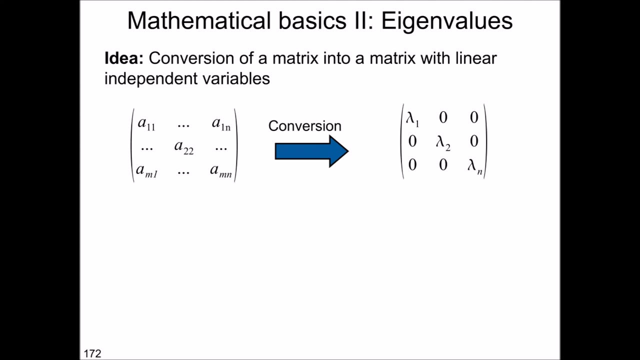 because this eigenvalue problem is the basis for many techniques in ordination and the multivariate real. so we proceed with the augen value problem and the idea is that a matrix is converted into a matrix with linear independent variables. so you have an initial matrix and afterwards. 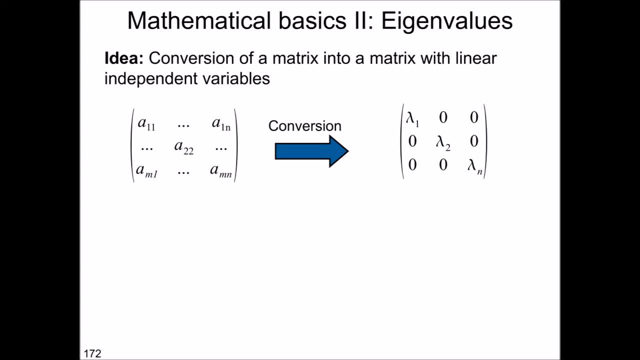 you have a matrix where the variables are linearly independent. that means you have only values along the diagonal. so we have encountered before that if you have, for example, would have the covariance of two descriptors in above or below the diagonal and this would be zero. then there is no relationship between the variables. 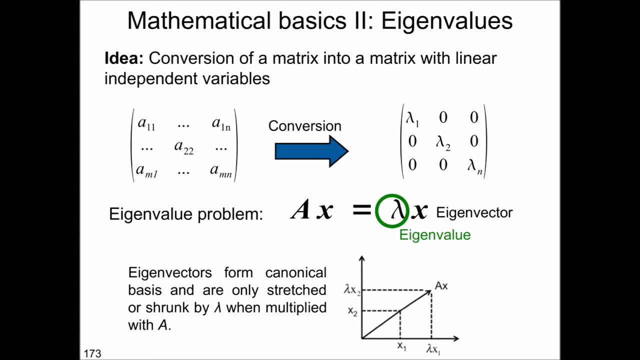 so the eigenvalue problem is generally written, as we have an initial matrix, a multiplied with the so-called eigenvectors and we obtain the matrix, and this is the same as the matrix of zeroima one. so this is pseud. Favorite again is of zeroessment order and the student will. 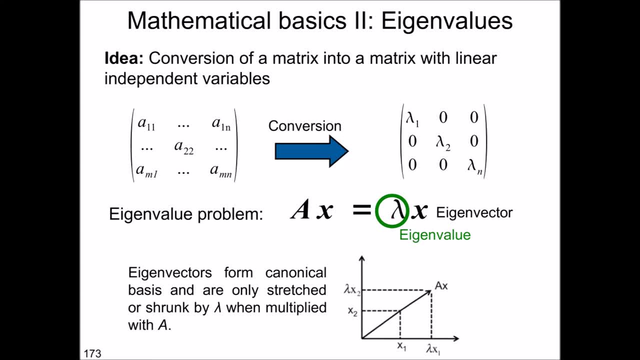 also do thechen shave for the matrix, and so you can. you can determine a matrix in caviar which is all�� height, so it would be the same way in unf spiral, and therefore of full hing height. but this is the 두�cho point. 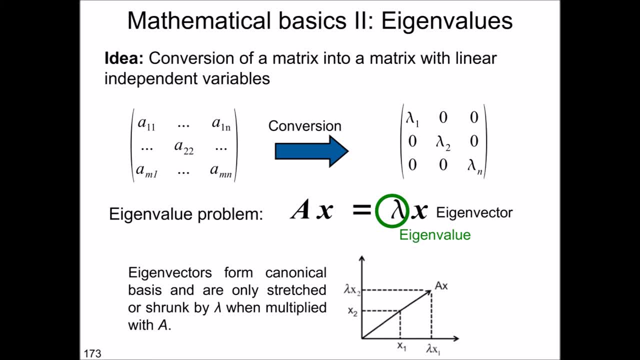 the intuited point, powder or theim, authentically, as we have seen we previous praj expansive examples of pure w to be bright. in other words, if we want to project some eigenvectors in these numbers, we have important z. interesting Walls point in a matrix a times a multiplied with x. so 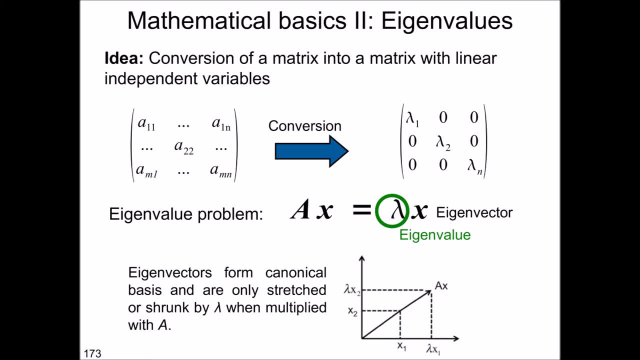 the eigenvalue problem can also be written as a linear function where we multiply the eigenvector with the eigenvalue and these vectors only stretched or shrunk, and this matrix of eigenvalues is called the canonical form, and that's what you encounter as term in many of the methods, for example canonical correspondence. 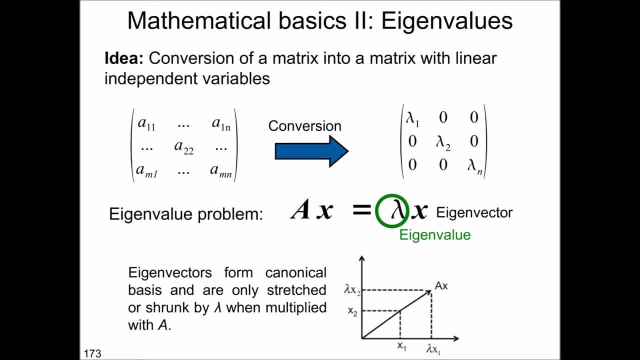 analysis, canonical correlation and so on. so geometrically, the eigenvector represents the rotation of initial coordinates in the in the initial coordinate system, and the eigenvalue just stretches the vector to its position. so on the no. in the notes to the slide you find a couple of examples of matrices, how they rotate. 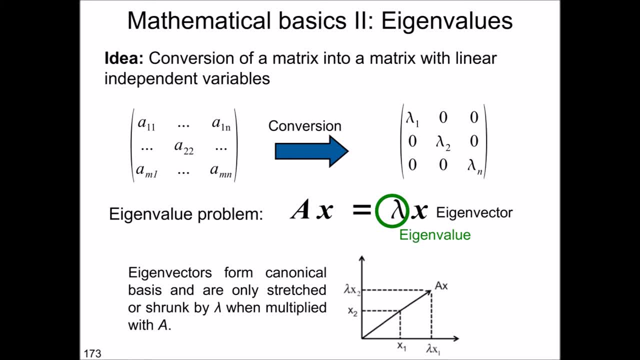 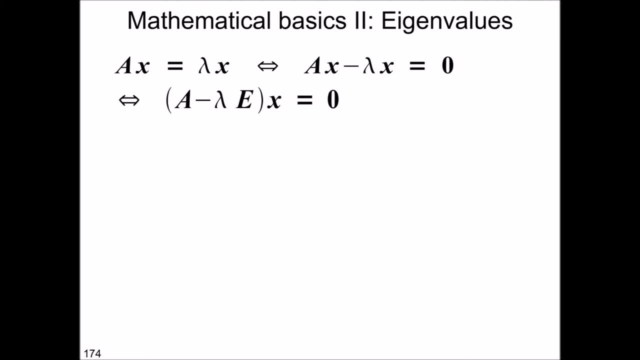 rotate or stretch different points with certain behavior coordinates. so let us reformulate the eigenvalue problem um. you see reformulation here in the equation. so we end up with the equation matrix a minus the eigenvalue times the identity matrix. so we ignore the trivial solution that x minus 와. 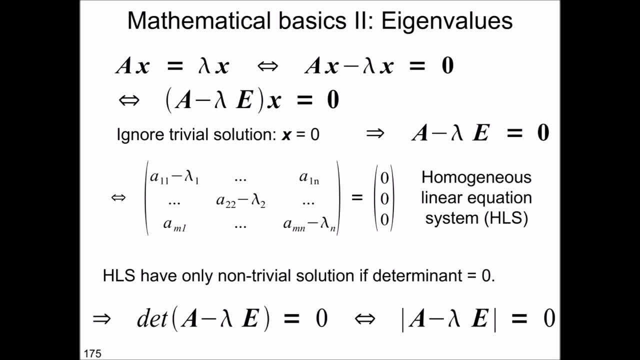 equals zero. this leads us to the equation: the matrix a minus the eigenvalues times the identity matrix equals zero, zero vector- and putting this into a different matrix form- rewriting. this is shown in the middle of the slide and this is a homogeneous linear equation system. now we know. 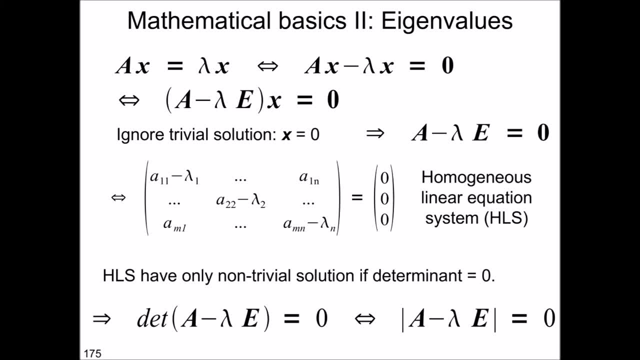 that for a homogeneous linear equation, system, um, and that this has a unique solution and that all x are the same and all are zero. and if this would be a singular matrix? singular matrix, at least one row is a linear combination of the other rows, so that means at least one x is independent from zero. 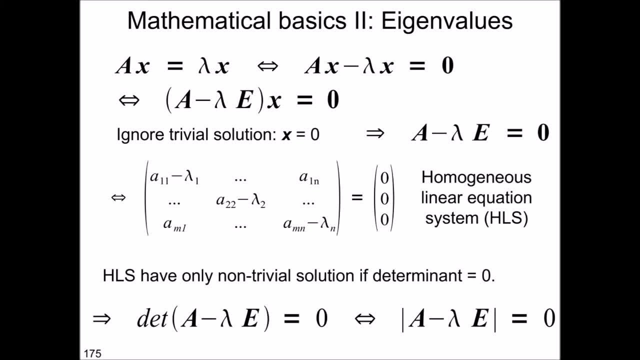 and in this case you don't have a unique solution. that means you can have enter different values for x, you just have relationships between the x- you don't have one unique solution- and the non-trivial. in this non-trivial case, the determinant is zero and 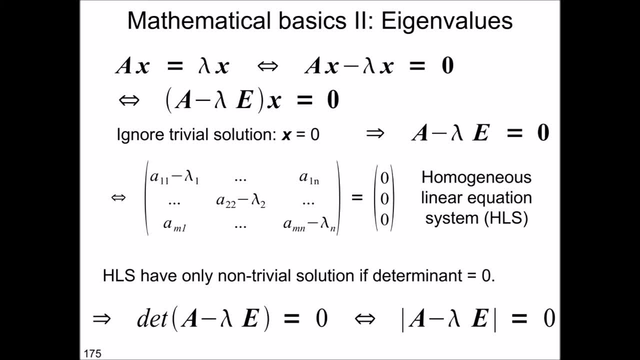 since we want to look for the case, or since we search for the case where not all x are zero, not all elements of the eigenvectors are zero. we look for the case where the determinant of the determinant is zero, hence the matrix is singular. this is shown um. that is shown in on this, in the last equation of this slide. 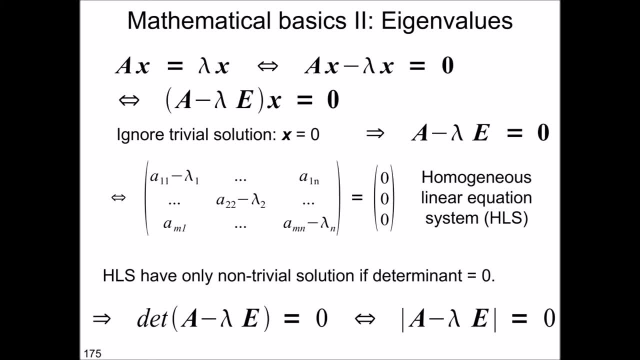 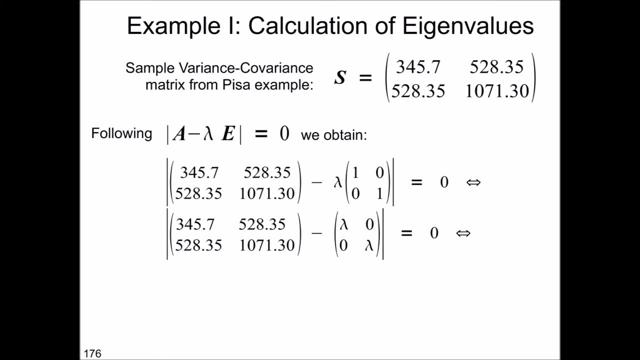 now let's look at the next slide. now let's look at the next slide. let's look at an example what this means to illustrate. so we have a sample variance covariance matrix from the pisa data, where we have the variances along the diagonal and we have the 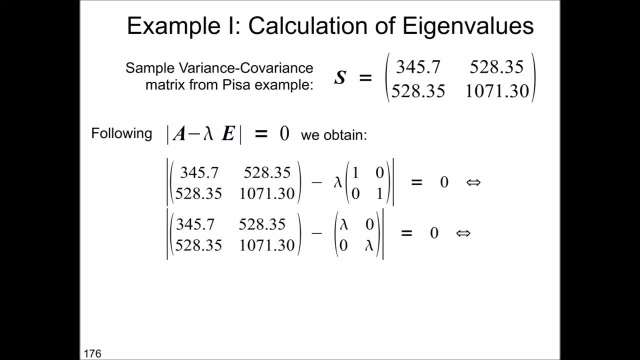 covariances given in above and below the diagonal. and when we now calculate the this um, then we have: when we want to calculate this, we have the matrix a, the variance covariance matrix, minus lambda times the identity matrix. we reformulate this to minus the matrix, the lambda in the diagonals, of course, in reality or in 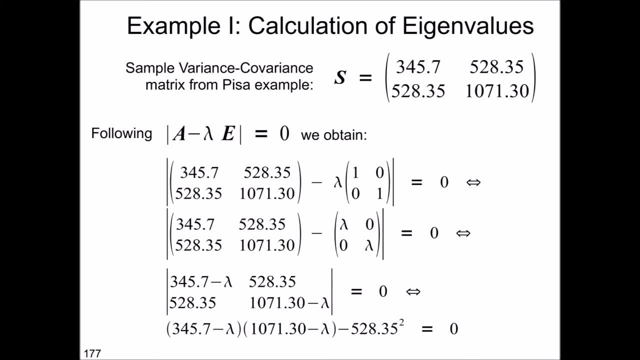 that's for the time being, just keep lambda here. so we calculate now um that we have to use this in this example. here we have u and z and we can see that the determinant of lambda is zero. now we have a space vector of delta and we can also 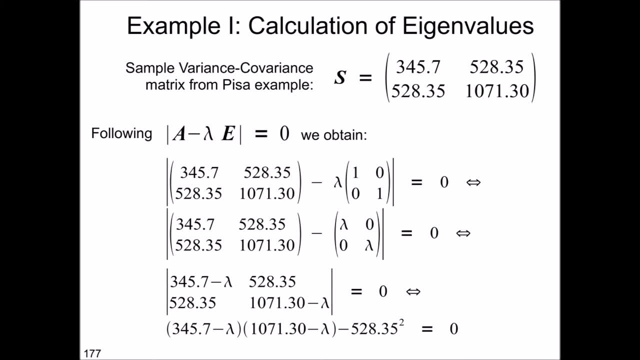 take down the determinant of lambda and we can separate it into the matrix calculation. so we have 345.7 minus lambda and 1000, 1071.3 minus lambda, and the determinant of that equals zero. now for for small determinants, we can calculate the determinant, the determinant, by hand, and it is done here for. 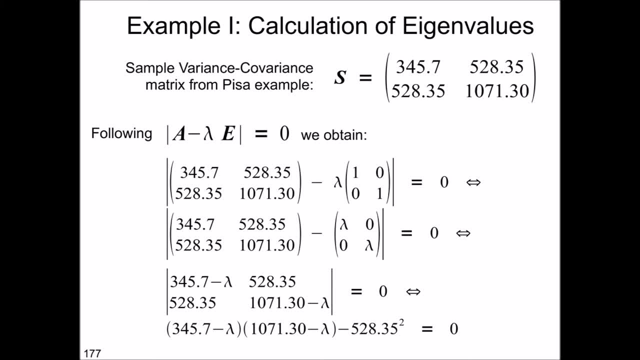 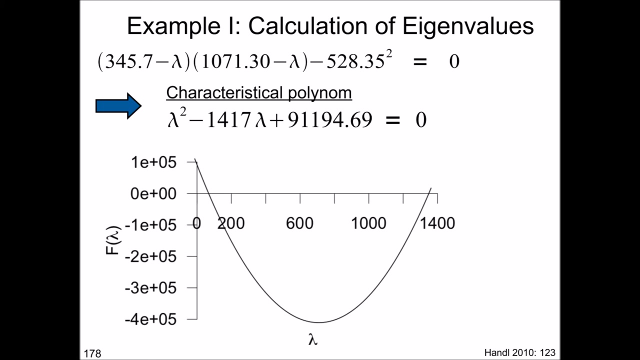 slide to understand what is a, b, c and d in our case, and this is shown here. so a times d is the first element, the top left element, multiplied with the bottom right element, minus minus b times c. so that means 528 squared. so we can reformulate this because this is basically a polynomial. 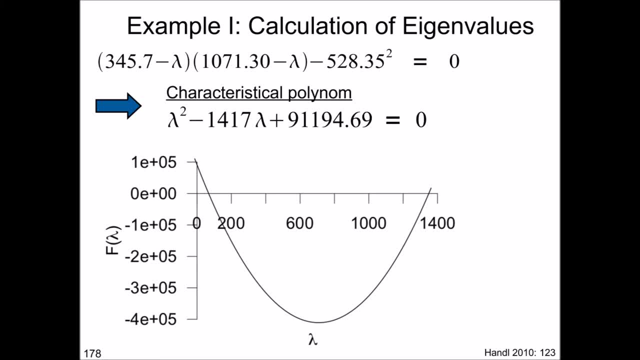 problem. we know that and this is research for the lambda- that means a bird's search for the solution for this equation for lambda and this is a quadratic equation and we know the solution from school for quadratic equations. we also know that when we can, we could plot this to find the solutions where we have the function of. 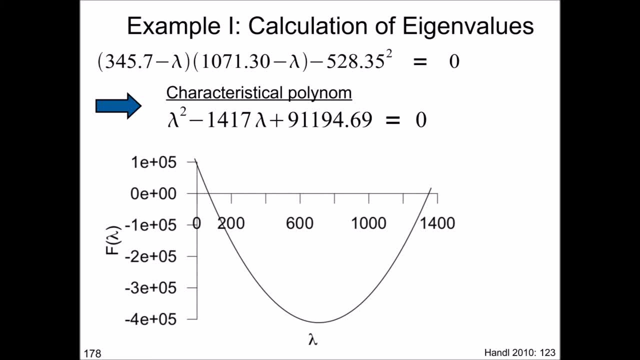 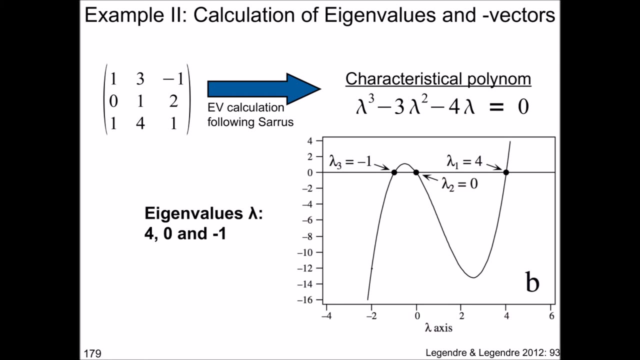 the number equals 0, so we obtain 2 Lambdas, in this case, that meet our conditions. in the next example we want to calculate eigenvalues and vectors and we start with this matrix that is shown on the top left of this figure. we all go in. 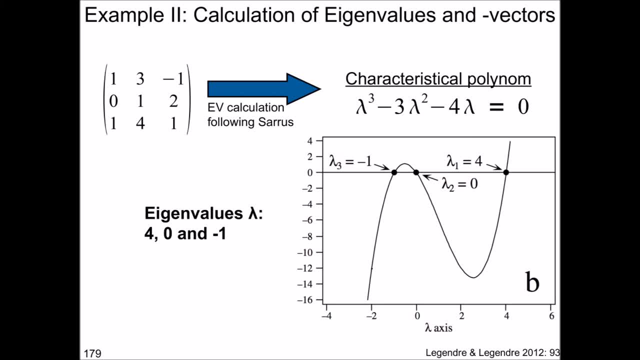 this way. we start with this matrix that is shown on the top left of this figure. we all go in to details here how we calculate the eigenvalues, but we can use the rule of Saru. you can look up this rule in a textbook or even a Wikipedia. we will 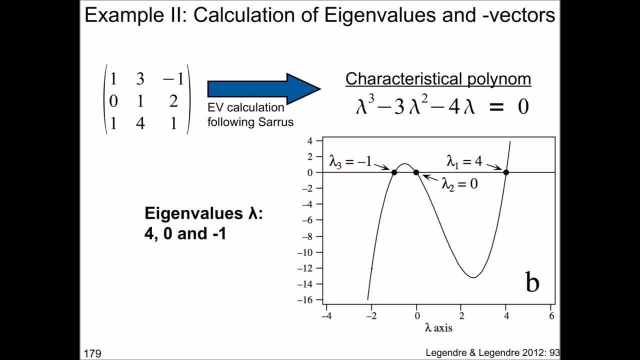 find this: how you can obtain the eigenvalues following this rule. this, this rule anyway, we have based on this matrix. you have the characteristic a polynome that is shown here and you have, you see in the figure. if you would plot this characteristic a polynome, then you would easily find out that the 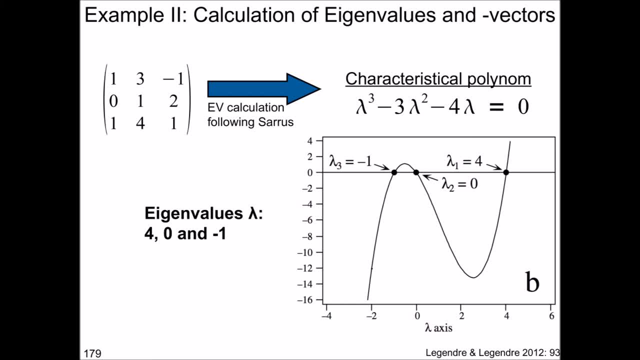 eigenvalues are lambda- 4, 0 and minus 1. you can. we can also see that this is rather an example. not for a real PCA, because we wouldn't have negative eigenvalues in a real PCA. you only have positive eigenvalues for a real PCA, because we wouldn't have negative eigenvalues in a real PCA. you only have positive eigenvalues for. 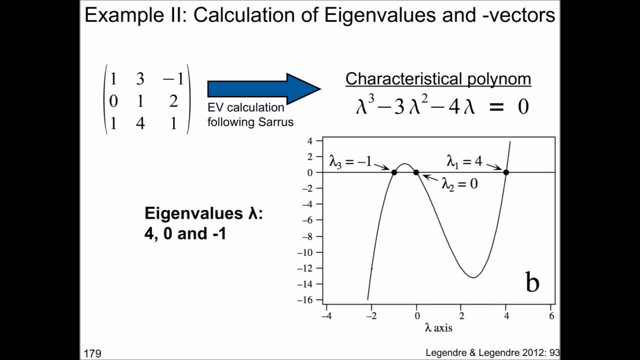 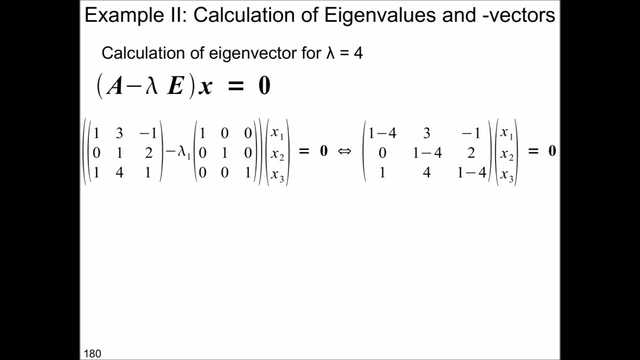 the individual axis. but this is just for illustration how the calculation of eigenvalues and eigenvectors works. so we calculate here: the eigenvector for lambda equals equal 4. so how do we do this? again, we set up the initial. we use the initial variance covariance matrix minus lambda times the identity matrix. 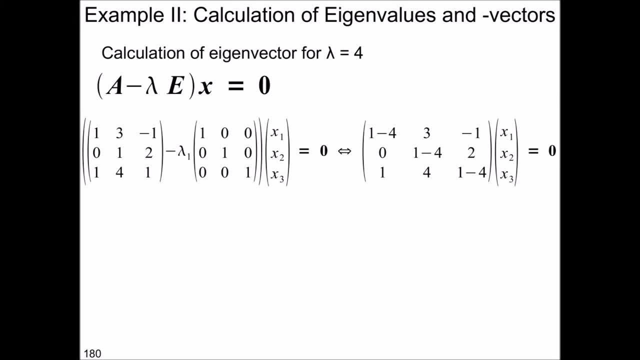 multiplied with X 1 equals 0. so we put in the eigenvalues and the eigenvalue is here 4, we rearrange and we obtain this equation system. so we know that if we would put X 1 equals X 2 equals X 3, then all X would be X 0. this would be: 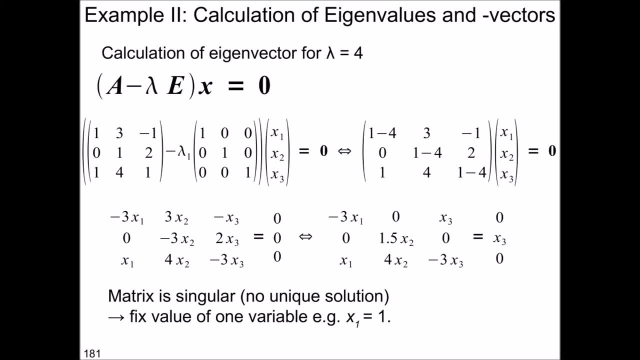 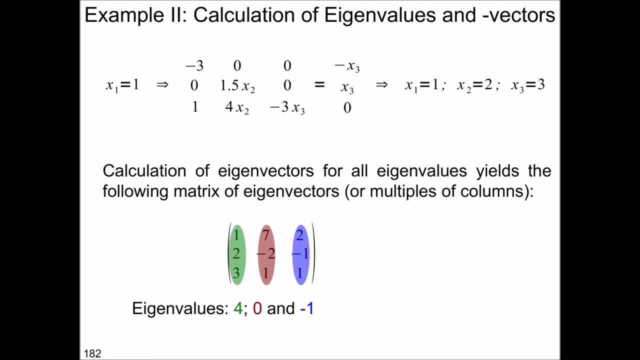 1 solution. so we ignore this. and we can do this by fixing the value of one variable. for example, we define X 1 n 1. so when we define X 1 s one, the equation system changes your scene in the bottom rod. now we have 1 plus 4 times X, 2 minus 3, X 3, because the other 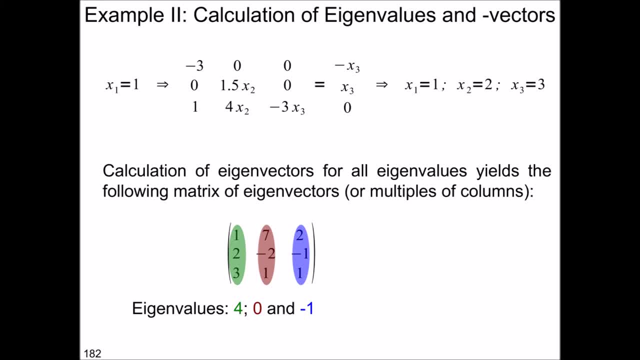 sausage, because if you take 1, then our bogus Stew. but it says the civilization pattern for that essentially is 0 Forest, and you take one base which is one positive new function, SP of Y, 1 plus 1, y minus y2. so we know this value, S is 1. 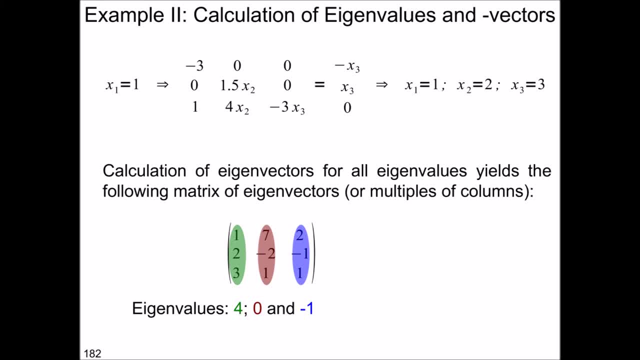 weise. so you can define as the later bracket and מצ editor one variable there, for example: et al. well, in that this of course should be here, one esemp three equals zero, and when we solve this equation system, then we obtain x one as x s one x two. 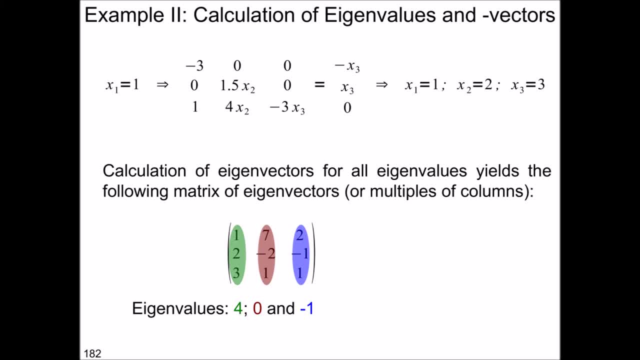 s two and x three s three. so this would be the first eigenvector for this matrix. so we have one, two, three as eigenvectors. note that in this time of this type of eigenvector calculation we ignore the condition that the eigenvectors the sum of the eigenvectors. 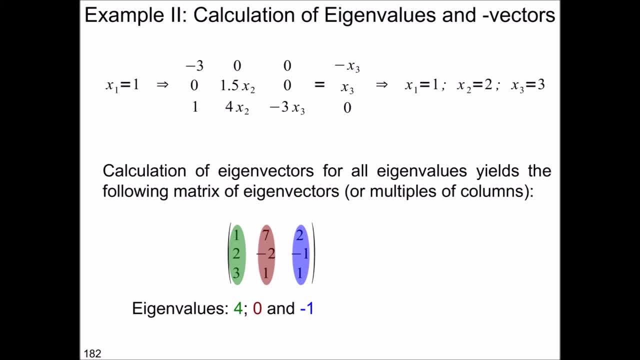 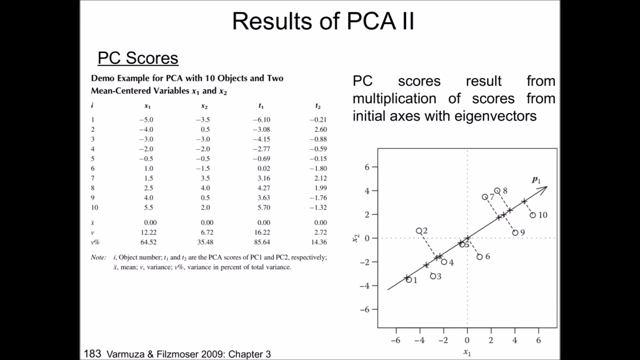 should be, should be one, and this is not fulfilled here. obviously, if you calculate the eigenvector, if you multiply the eigenvector with the transpose of the eigenvector, that does not yield one. so now that we know what eigenvalues and eigenvectors are and have a basic understanding, 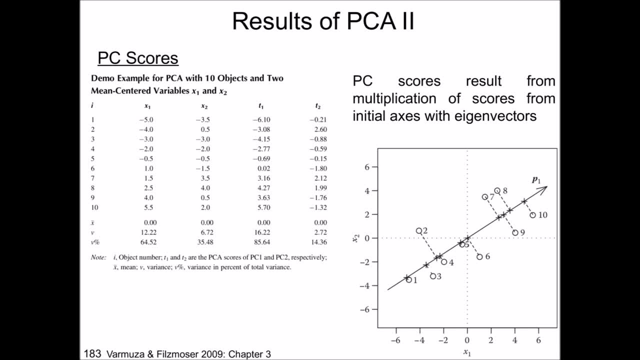 of the eigenvectors. we can now calculate the eigenvectors of how pca works. we look more into the results of the pca and something that you obtain are the so called pc scores, the principal component scores, and these show the positions of the object, the new scores of the object when on the new, on the new components that we have derived. so, on the new, 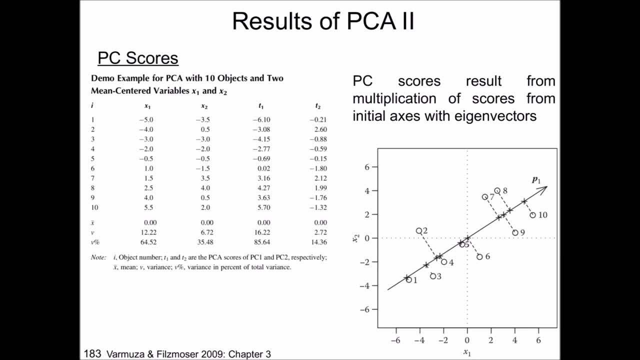 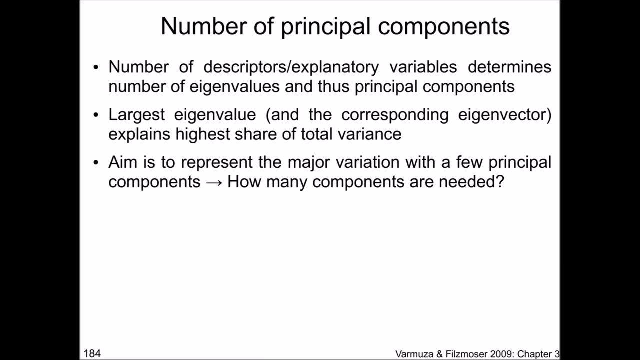 axis with maximum variance, and these pc scores result from multiplication of the scores from the initial axis with the eigenvectors. so how many principal components do we typically have? we've already discussed that this depends on the number of descriptors or explanatory variance variables- whatever you have in your data set- and this will yield the number of eigenvalues and thus 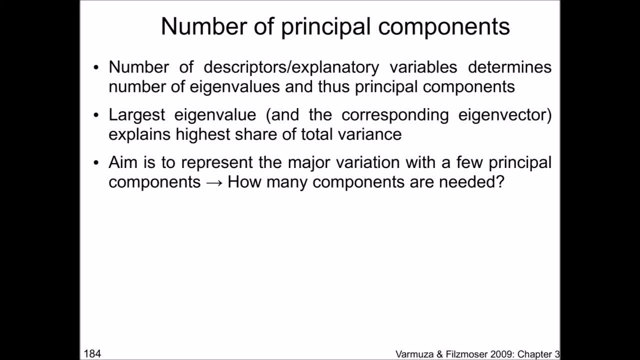 principal components. so the largest eigenvalue and the corresponding eigenvector explain the highest share of total variance, and that will typically be the first axis or the first component. if the aim is to represent a major variation with a few principal components, then this leads us to the question: how many components? 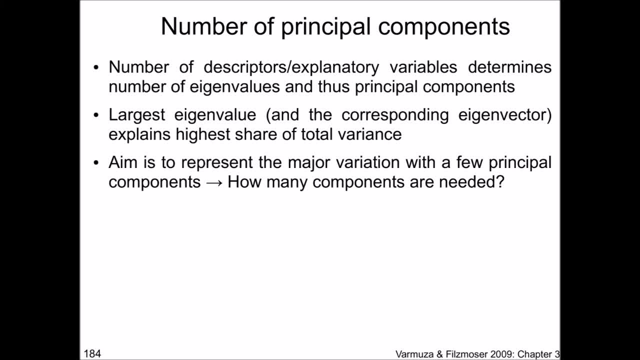 are needed and on the figure you see a couple of examples how many axes you would need for different data. you so you see that if the data is completely scattered around three dimensions- that's the figure to the left- then you also would need three relevant component. If all the data is in a plane- that's the middle figure- then we only 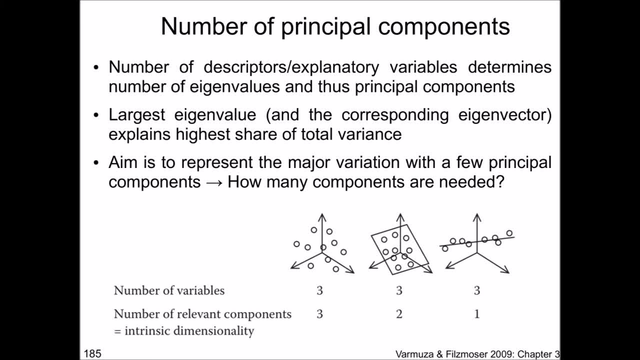 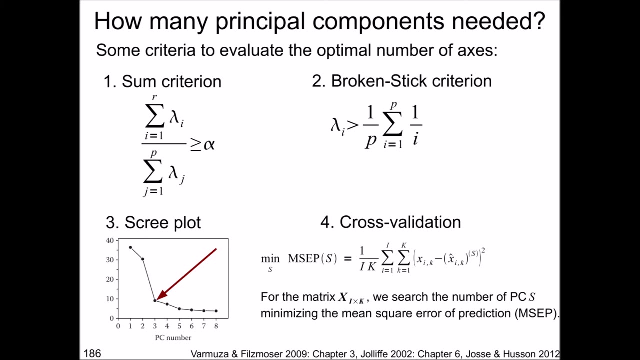 would need two components, and if they all are on one line, then you would only need one component to represent a major variation of the data. So we somehow need a criteria to evaluate the number of components that we need. So let us discuss some criteria that have been developed to evaluate the 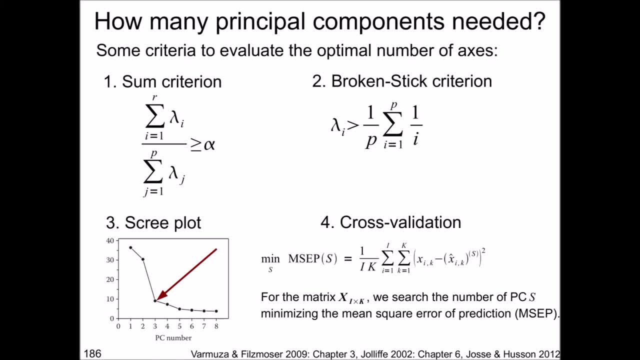 number of principal components that are needed, And one of these criteria is the sum criterion. Or note before that there is no single accepted criterion that works under all conditions, because it also depends why you are doing a principal component analysis. or there is no single accepted criterion that works under all conditions, because it also depends why you are doing a principal component analysis or similar analysis. 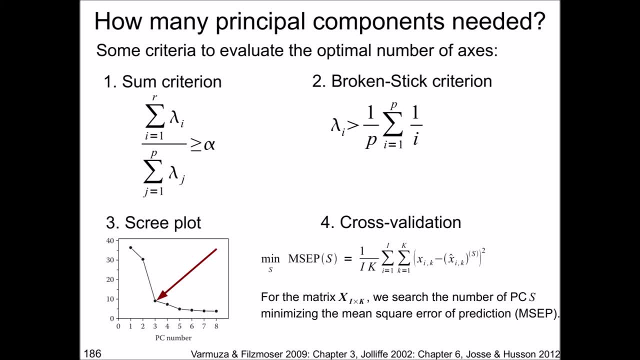 so if your aim is prediction, let's say, or principal component regression, then the sum criterion may be acceptable for you, because you want to know how much of the original variance is captured by the term, by the selected number of components, and to do this you set an alpha. 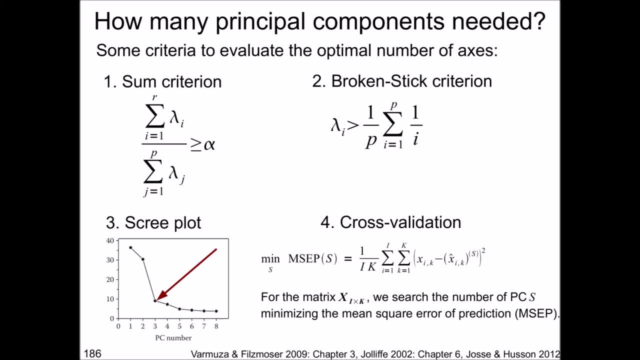 that gives the number, the proportion of cumulative variance that you want to preserve, and the sum criterion tells you how many of the principal components you may, you may, you need to keep to arrive at this amount of total, of this fraction of cumulative variance. for example, you could set an alpha of 0.9, which means that you would take 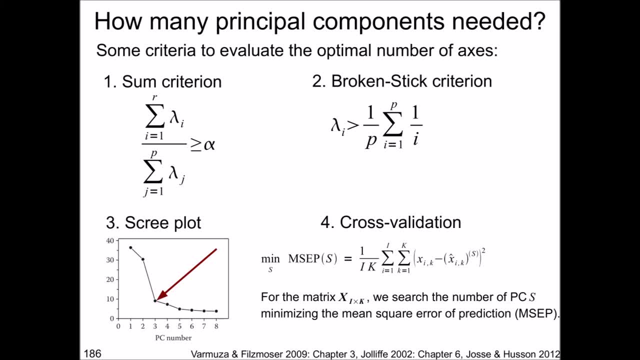 as many principal components that are needed to to capture 90 percent of the original variance. typical typically value between 0.7 and 0.9 is chosen for alpha. however, the optimal alpha will decrease with an increase in the number of variables in the data set. 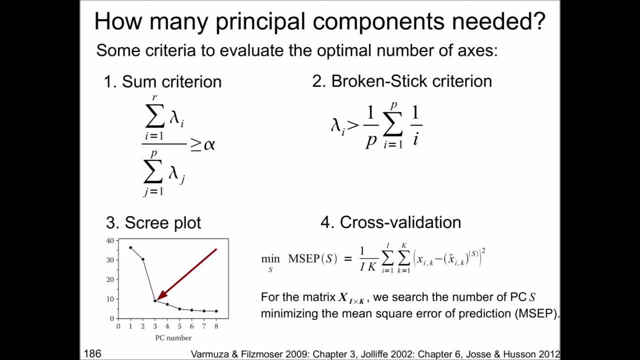 anyway, this is more a you heuristic criterion or a criterion that is ad hoc set. another criterion that has foundation or it is theoretically motivated is the broken stick criterion. it's the second criterion here, where you imagine that you have a stick of unit length and you practice in a 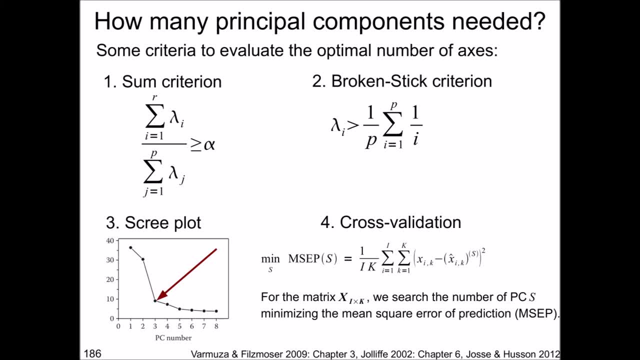 couple of pieces many times, and then the amount of variance that is provided by the, by the individual, when the resulting pieces is sorted in decreasing order and you compare the size to the eigenvalues from this broken stick model. so you can read a little bit more in the in the notes to this slide. i don't go into detailed explanation here, just 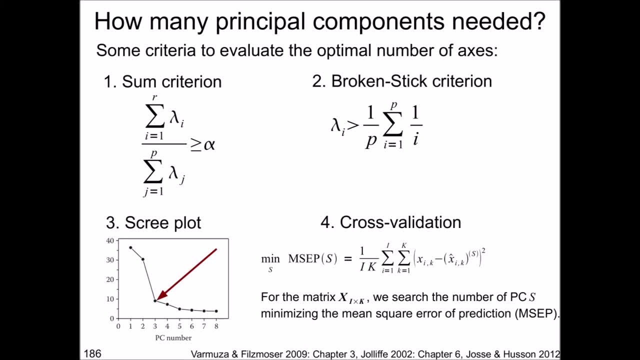 one motivated one different way of drawing. is it contractors? when the value in real beggar or see things thing, 0.5 on and the other one in infinitely small, so on average we obtain is a breaking point at 75 percent? you can see that if you do the calculations. so what does this mean if we had two variables in 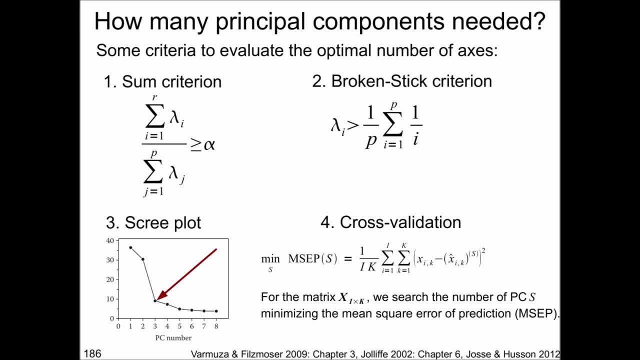 our pca. we would say by: if we just break random the variance, then 75 percent would be on the first axis and 25 percent on the second axis. and if our variance for the first axis is smaller, then we would evaluate that a random variable would yield more variance on the first axis. then and and then. 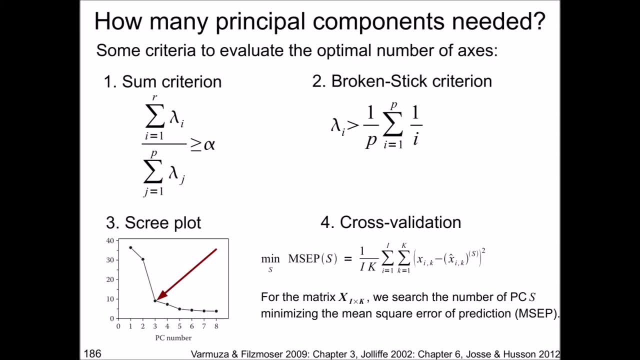 it's perhaps not meaningful and we don't need to keep that component. then we have the scree plot and the scree plot where we would display the variance on the product table. in the previous we look for an elbow point. So scree is the rubble from some. 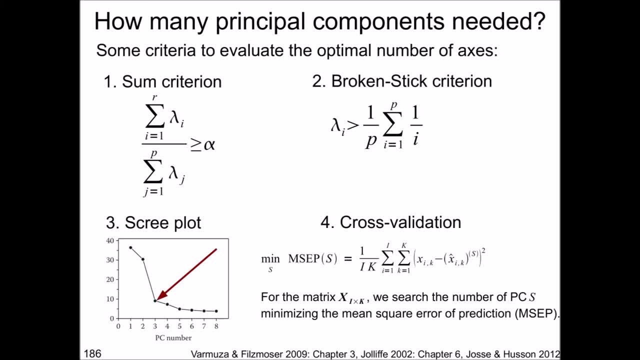 if some stones fall down from the cliff then they build up as rubble And in a scree plot you search for the beginning of the scree, of this rubble that piles up at the bottom from the cliff. So you search for this largest drop. 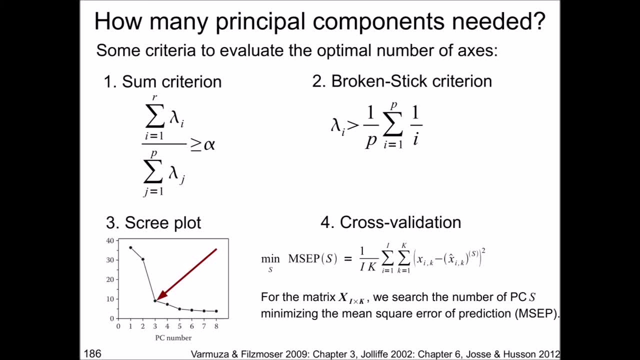 and it's indicated with the arrow where this largest drop would be. Again, this is rather a subjective technique, because you may also argue that the PCE number five. you would evaluate that the scree begins. So it's rather a subjective criterion. 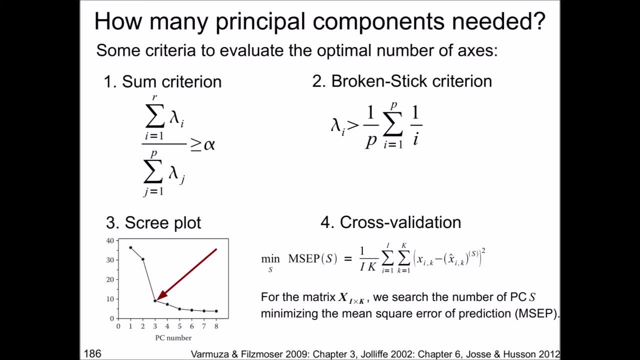 So a more objective criterion is finally, cross-validation, where we minimize the mean square error of prediction that's shown here. So we remove and cross-validation. you already, we've already discussed this. We remove from the matrix different values and we use- we later on predicted- these values. 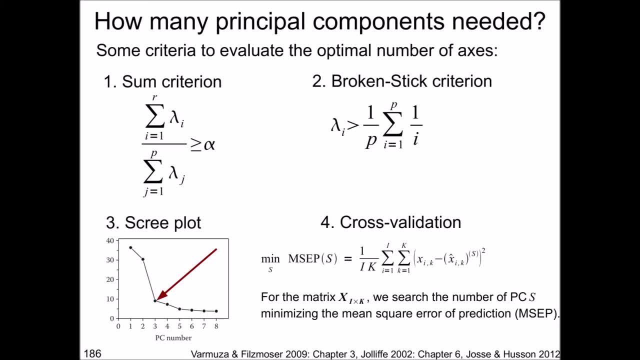 based on our principle component analysis And this is then for different number of principle components. this is done And we average here by the number of the average, this for the number of principle components. If we do this multiple times and we search for the number of principle components, 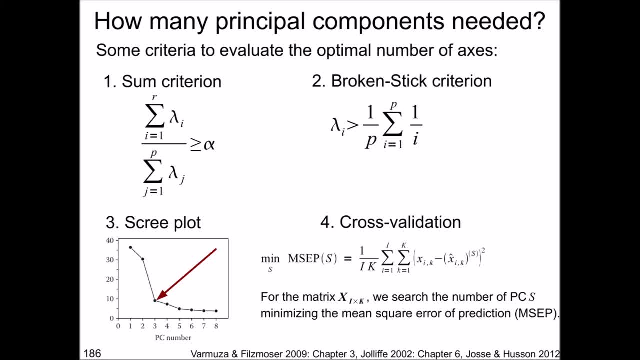 that minimizes this mean square error of prediction. There are also some statistical tests, but they are in many cases less reliable than cross-validation And they are sensitive to deviations from the multivariate normal distribution. So we don't discuss them here in the course. 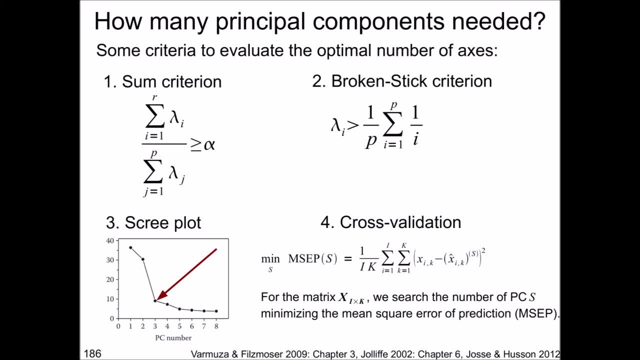 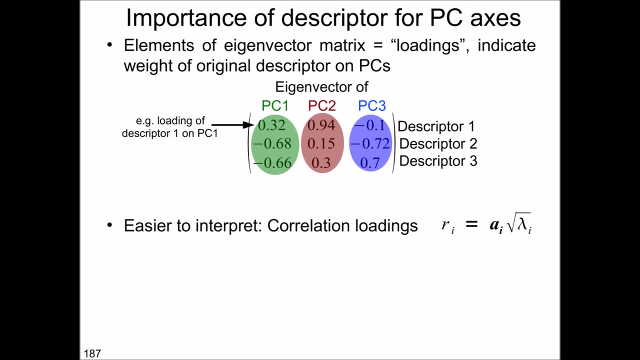 but you can replay it to the literature to look into more into the details. So now that we know how many components we need, we need to discuss, when we have our results, how we can evaluate the relevance of the initial descriptors or variables for the different principle components. 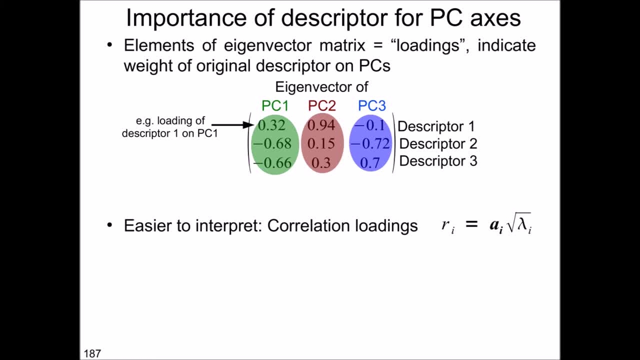 This is done, or this is evaluated, based on the eigenvectors, because the elements of the eigenvectors are the so-called loadings, And I have displayed on this slide the eigenvector matrix for a case of three variables. As a result of the whole analysis, 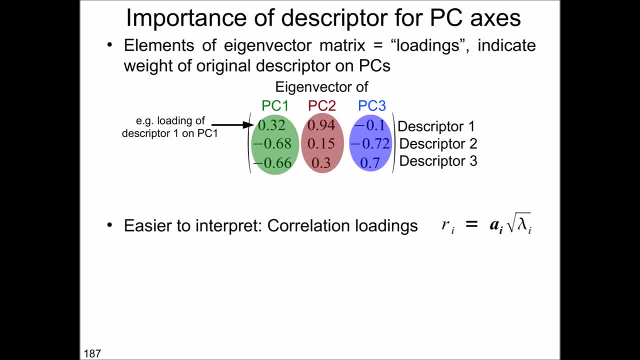 you would have these matrix of eigenvectors for, and they stand for the eigenvectors on PC1, and they stand for the eigenvectors on PC1,, PC2, and PC3.. And each of these elements of the eigenvectors for PC1. 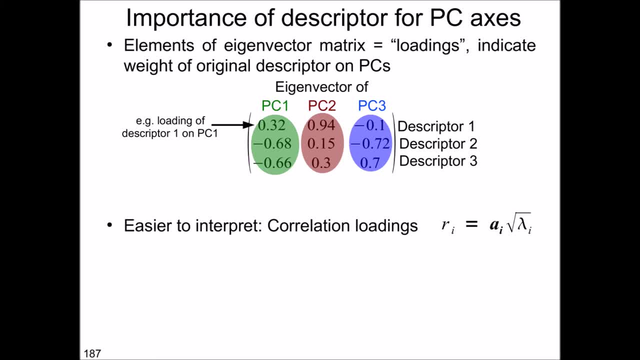 would be the loading of the descriptor one, two and three. So they represent the weight of the original descriptors on the PCs. So, on relative or in relation to each other, you can interpret the weight of the different descriptors. However, if you want to have a more easier way, 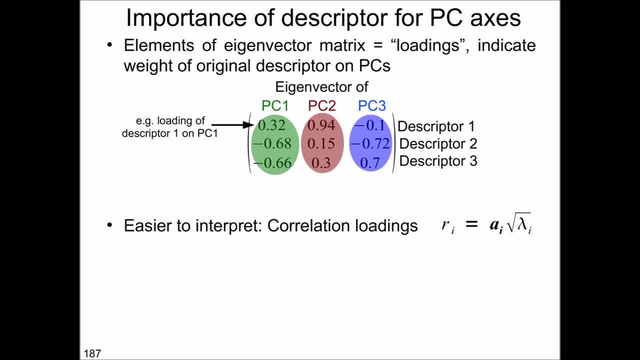 to interpret these is to obtain correlation loadings, And correlation loadings are obtained if you multiply these eigenvectors with the square root of the eigenvalues. Well, note that correlation loadings are equivalent to correlating the original descriptors with the PC scores. 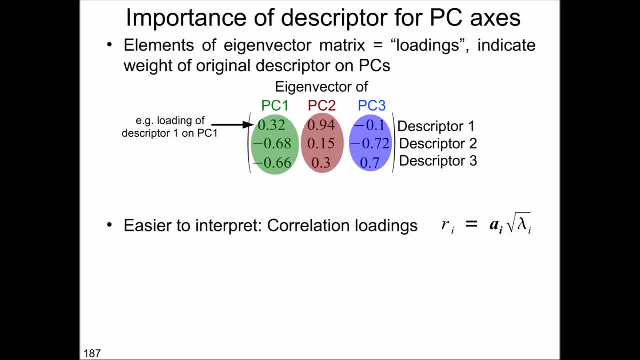 And note also that the term loadings is used differently in textbooks. So some textbooks use loadings for this correlation loadings and whereas in our loadings are basically the elements of the eigenvectors. One problem may be that if you have many variables, then more or less all variables may contribute at least to a small extent to each of the principal components, and that makes the interpretation very difficult. 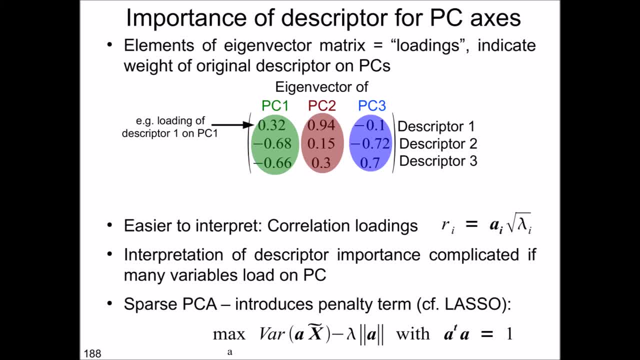 For example, let's say that we have six or seven variables, Principal components and variables- and each of the variables contributes a little bit to each of the axes, some more, some less. So how do you interpret then the individual axes? It is relatively difficult if you have many variables, and in the R case example you will see this for the case of 14 variables. 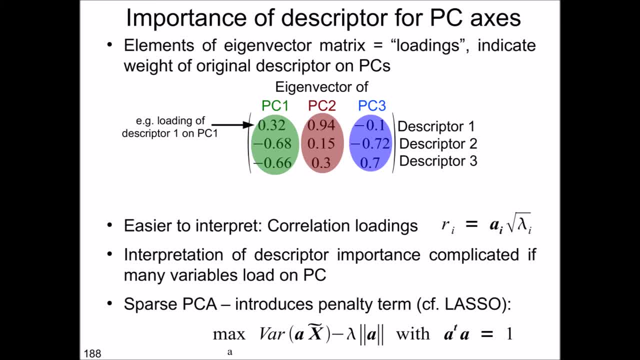 So one solution is here: to conduct a sparse PCA, and this introduces analysis. This is a penalty term to the maximization problem that we've already discussed. This is a similar interpretation as for the lasso that we have discussed in more detail in the course before in the context of multilinear regression analysis. 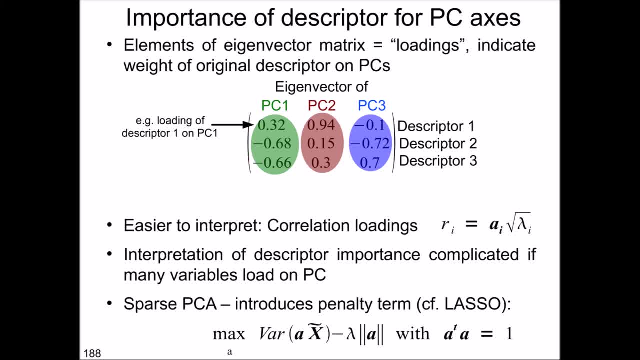 So the motivating idea is that we set a penalty on the size of the elements of the eigenvectors And basically, we want, We want to shrink some of the loadings to zero and increase the loadings of others, and this equals that, or this means that in the end we have some descriptors that play no role because the loading becomes zero, whereas other descriptors become and gain a higher weight. 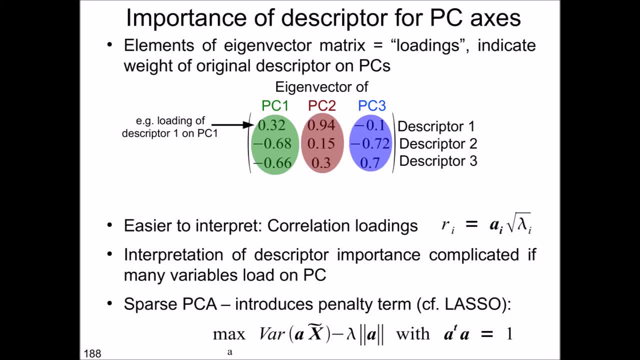 So this is somehow clear. It's called sparse PCA and this is used if we want to have a clearer Interpretation of individual principal components, for example, if we use them in follow-up analysis. For more details, refer to the notes to this slide and read the literature. 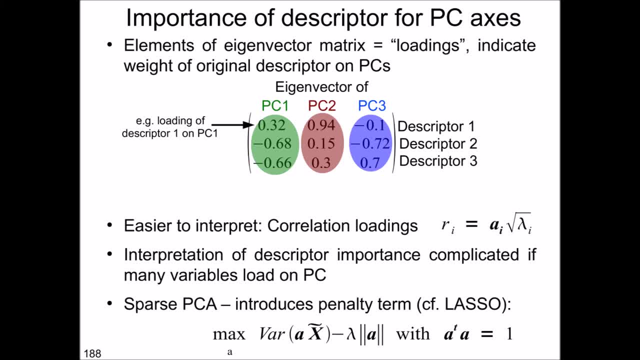 Note also. I mean the Note also that the lambda that is used here in the penalty term in the equation Maximum variance of A times the transformed and centered matrix X minus lambda Times. this is this lambda is not an eigenvalue. that is very confusing here in the context of PCA. but we have to stick to the terminology. 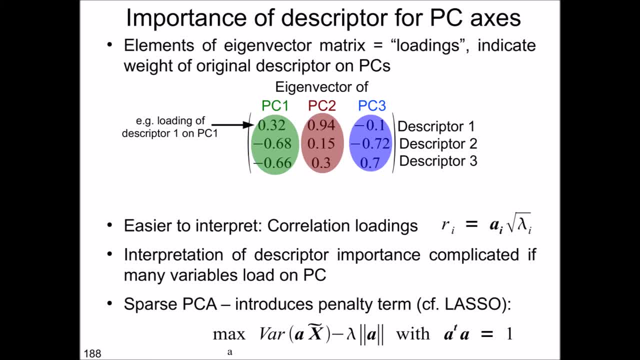 This is used in the papers. It's called. it's the lambda that is optimized, the lambda penalty that is optimized, and you know this already from lasso. but don't confuse this with the lambda. and that is used for the eigenvalues. That's also. 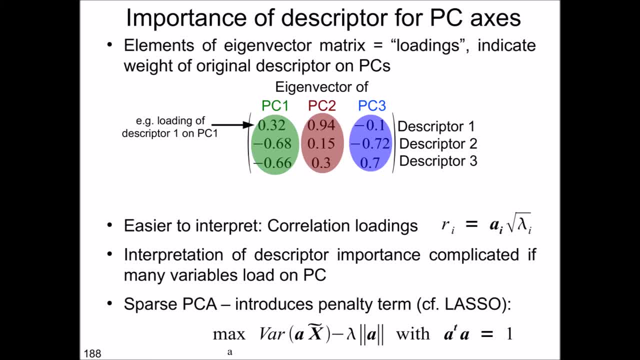 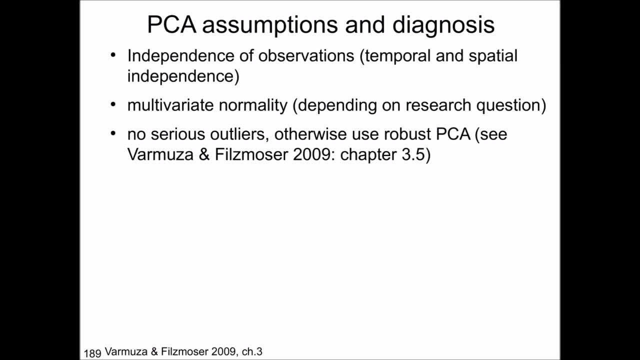 The result of a maximization problem. We turn to the PCA assumptions and diagnosis. So the assumptions of PCA- were, are, and that's known from other data analysis methods and Unifroid case that we've discussed before- Is that the Observations are independent, so that we have temporal and spatial independence, that we that we have multivariate normality. 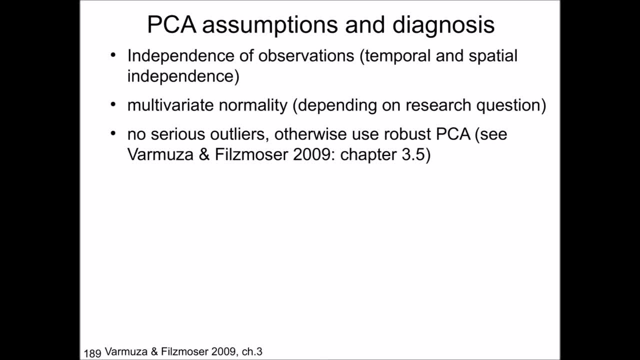 Although this assumption is not required for all analysis. For example, it is not required if we only want to visualize the, if you only want to visualize the data, This can be done reliably, even for discrete Variables, as long as the database on numerical and the distances between the discrete values meaningful. 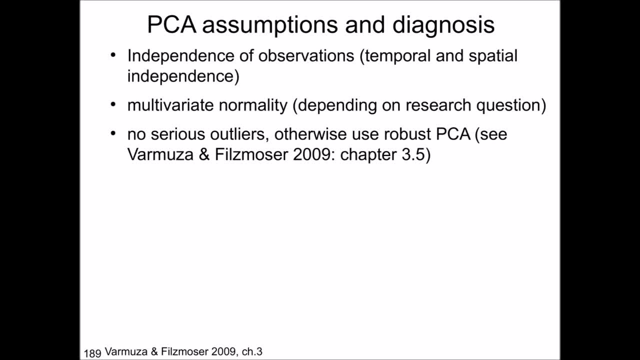 If you use it in regression analysis- the results of the principal component analysis analysis- then multivariate normality is required and many hypothesis, math methods, testing methods, would also require multivariate normality. Another assumption is that we have no serial Serious outliers, Otherwise you can use the real robust PCA. 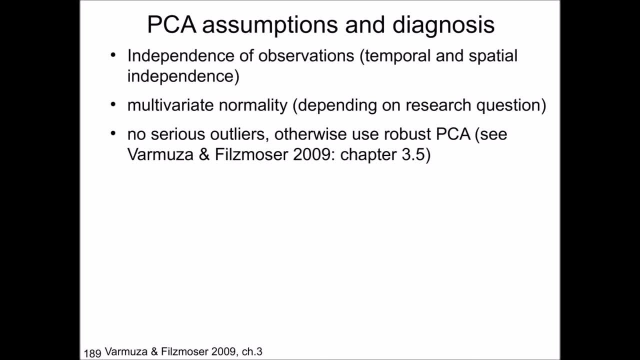 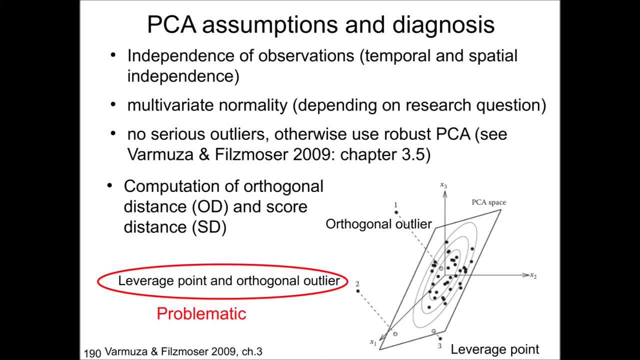 In fact, in the course we mainly use the robust PCA. If you want to read no more details about this, read chapter 3.5, and one was and fills Moser. So in the context of multiple linear regression, we discussed leverage points. 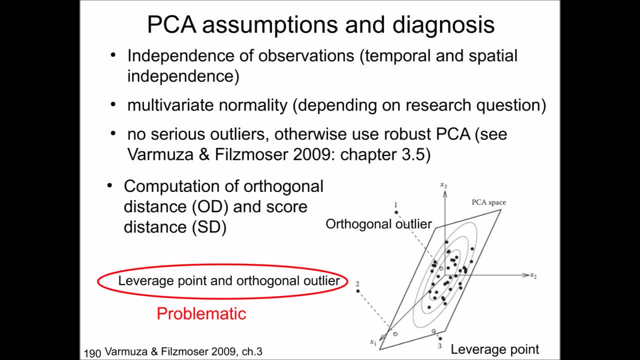 And and outliers from the model And we have something similar in the space of the, Of the PCA. we have, on the one hand, We have score distances that are something like leverage points. These are just very different in the scores and in this space and the distance to the other objects. 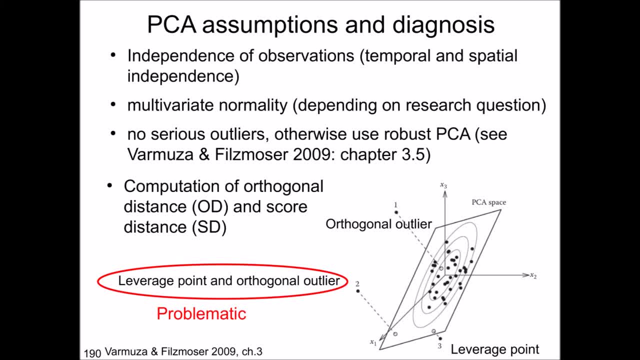 So they may have a higher Weight in modeling. and we also have orthogonal distances. That is the difference to the PCA space, and these orthogonal outliers are displayed, as well as deviation from the PCA space, in in the figure And, as we discussed before, leverage points- if a point is a leverage point, 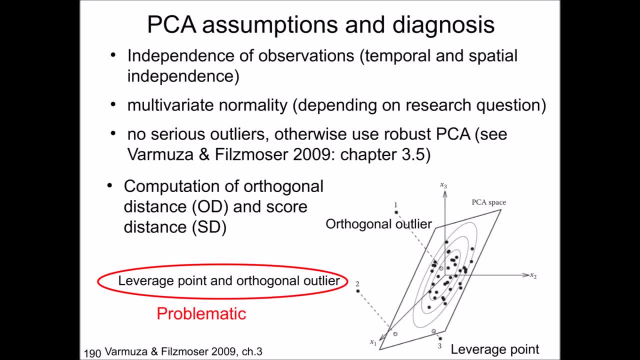 And an orthogonal outlier, then we have may have a problem and these are most problematic points, Or these are, they are more influential than other points and we should remove them and repeat the analysis. However, if you do a robust PCA, this will in most cases not really matter. 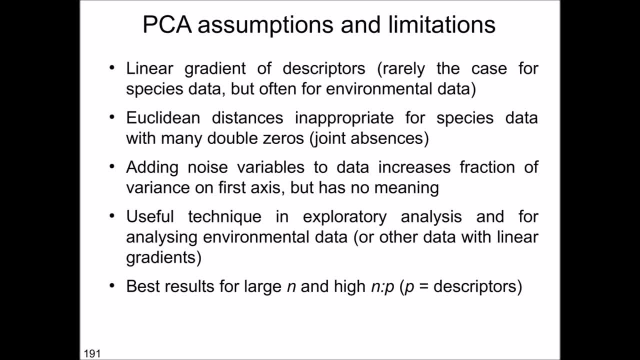 Yeah, generally the PCA also assumes that you have a linear gradient of descriptors. This is rarely the case for species data, Although you can transform the species data, for example by Hellinger transformation to a key, to a key linear relationship, But in it for environmental data, for example. 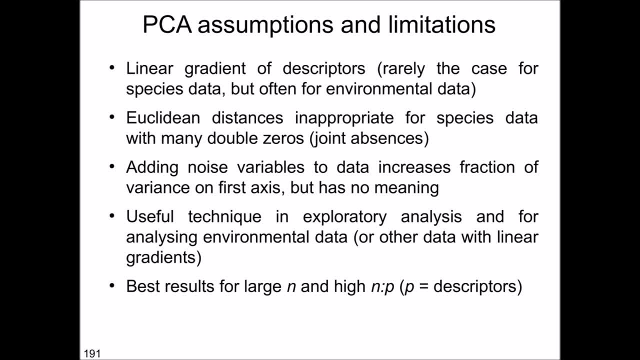 Yeah, that's the soil data That We use, or other environmental variables that this is more of, given that we have a linear gradient of the descriptors. Euclidean distances are often inappropriate for species data because you have many double zeros, So joint absences are very often occurring, and we will discuss this later on what this means. 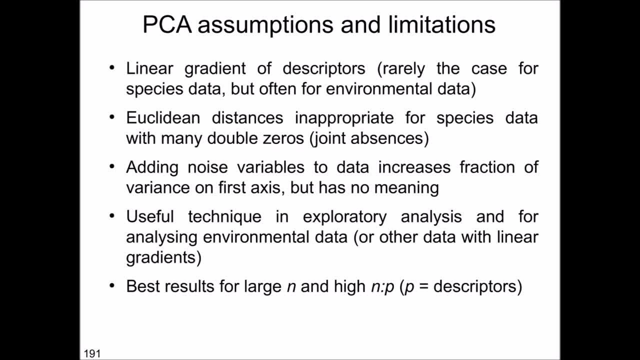 Why this is inappropriate in the context of distance math, math measures. and One additional problem is that if you add noise variables to data, this increases the fraction of variance on the first axis, but this has no meaning. It is overall a useful technique and exploratory analysis and for analyzing environmental data or other data with linear gradients. 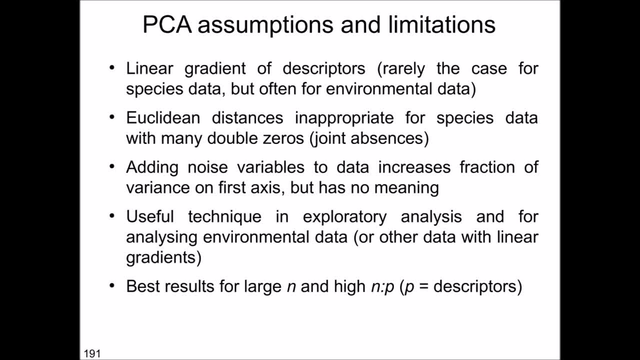 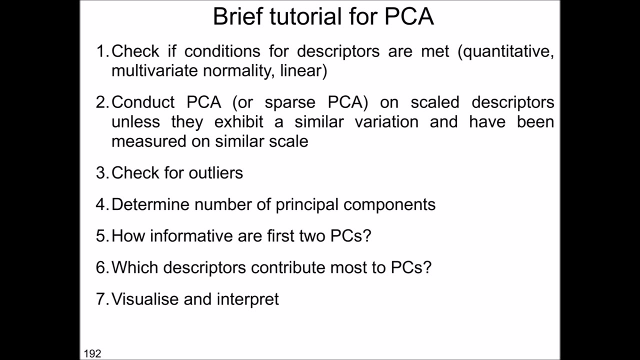 It helps you to display the data and you obtain the best results If you have a Large and and high and to P ratio. but it is not surprising that holds actually for many methods. So we look at the brief tutorial for PCA first. you check if conditions for the descriptors are met, depending on your research question. 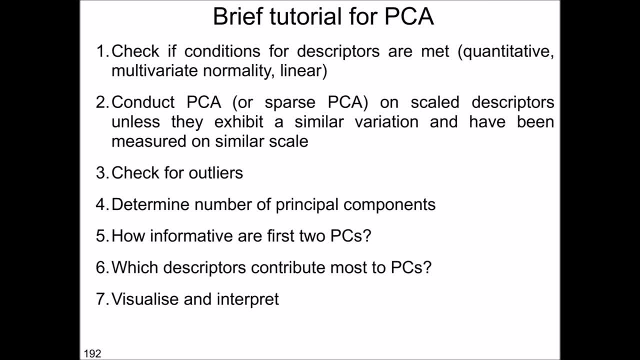 You conduct the PCA, or sparse PCA, on the scale descriptors, unless they exhibit a similar variation and have been more heavy measured on the same scale. Then you check for outliers, You determine the number of principal components and you evaluate how informative the first two PCs are, because it's important to know when you plot the data. 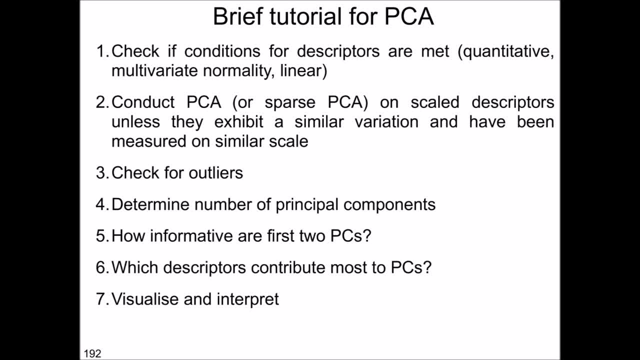 For example, in the B, plot on the first two components and then, Depending on your, what your interest is, you may evaluate the contribution of individual descriptors to the PCs. and finally, yeah, plot the PC, Perhaps with the descriptors, and interpret the results, what you see, or extract, and afterwards perhaps extract. 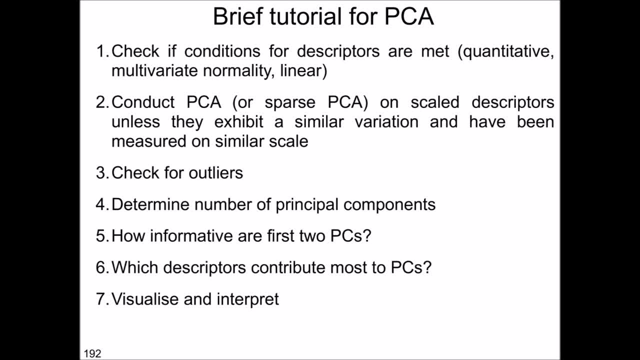 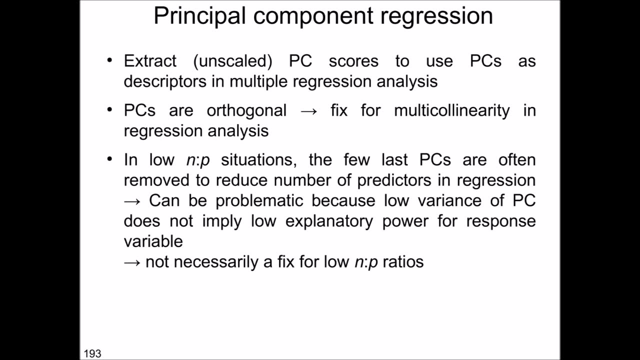 The scores for principal component regression and that's discussed as Last Aspect of principal component analysis. The last topic we discuss in the context of principal component analysis is principal component regression. We've mentioned this term a couple of times and this is the last issue we want to discuss here. the idea of principal component regression is that first, 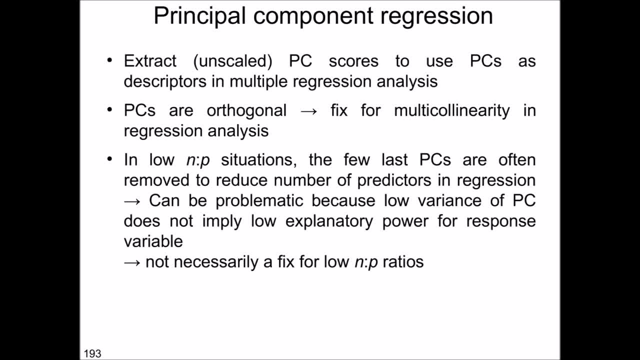 You use the descriptors- a principal component analysis, and then you extract the unscaled pc scores to use these as new descriptors and multiple regression analysis. but why should we do this? the motivating idea is that if you have multi-culinarity among the variables, then this can be fixed because the new 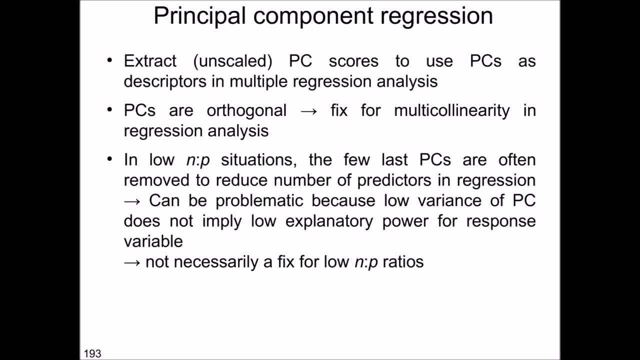 principal components that are extracted are orthogonal, so they are completely independent from one each other. you don't have any problem with multi-culinarity anymore. in addition, if you, if you use, for example, the sparse pca, you may extract gradients of joint variables that are so principal components that are representative for a couple of variables that represent more. 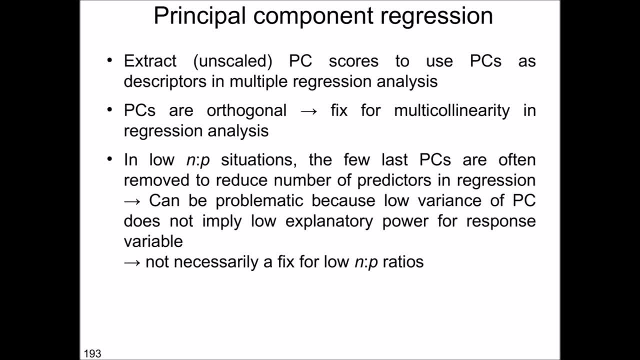 meaningful gradients, for example gradients of water quality, where the variables, where the initial quality variables, such as ph, oxygen content and so on, are correlated with these and the other principal components are can be interpreted for other environmental gradients, for example in terms of, in the given example, of water quality, water quality gradients. on the one hand, this can be: 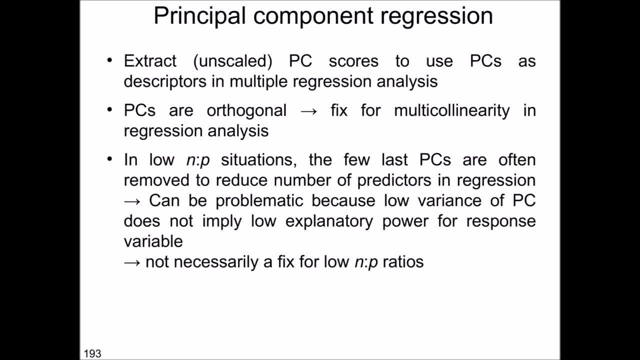 habitat gradients or climate gradients or something else. often these principal component regression is also used in the context of low end to p situation, so when you have relatively low number of samples or observations per parameter in the model, because if you remove the last principal components then you can reduce the number of predictors. so, for example, 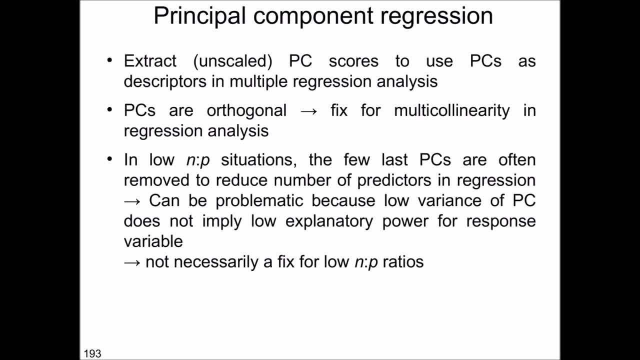 you keep only the principal components that explain 90 to 95 percent of the variance and you remove the other ones, and then you have a lower number of predictors in your multiple regression model. well, this is often done and seems appealing. the problem is that the law variance last pc's, so the